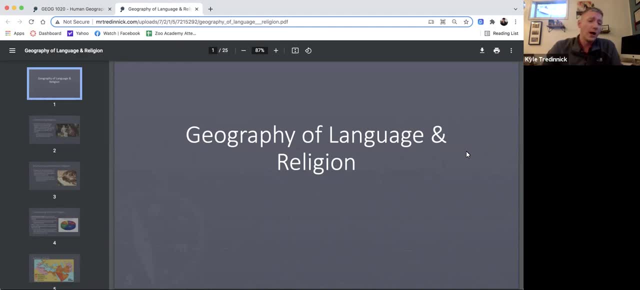 documented, so much information out there and so relatable to students that they're really great in terms of being able to connect these ideas of cultural diffusion, cultural hearths, to things that we can see very clearly on multiple scales. So we can look local, national, international, and then we can look space and time. 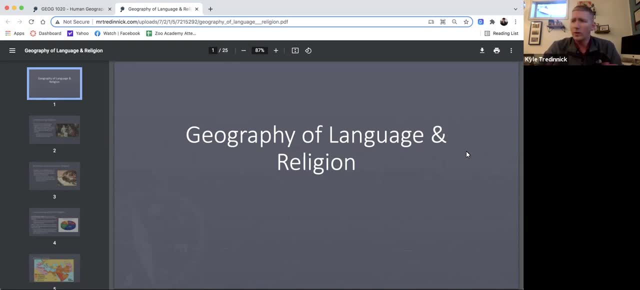 So getting right into it. one of the things that I'll also say about this is that, again, just the disclaimer is not trying to dissuade or persuade to any political or not political, any certain sets of beliefs, but just kind of saying: here's what they are, here's how geography focuses on it. 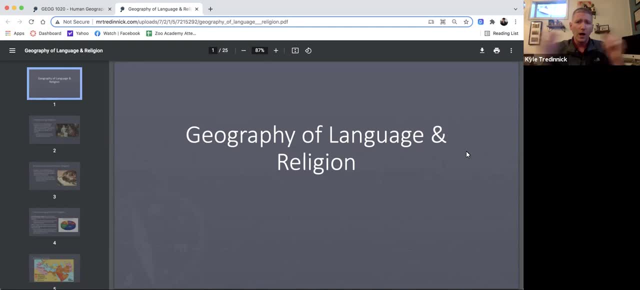 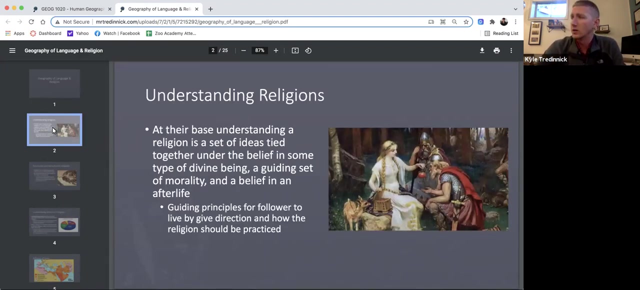 So I'm not trying to favor one religion or one language even over another, But just saying here's geographically how we can track these over space and time. So, that being said, definition of religion, and there's key aspects of religion that really distinguish between religion and philosophical sets. 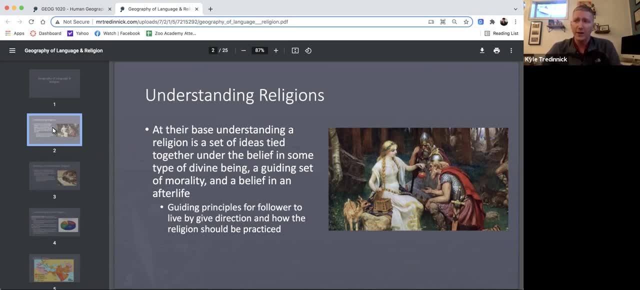 So there is a difference when we're looking at what all does religion, what do religions have in common? and again, not trying to put one over another, but, um, what we're seeing with religions is they all have some sort of divinity, some sort of understanding of a divine. 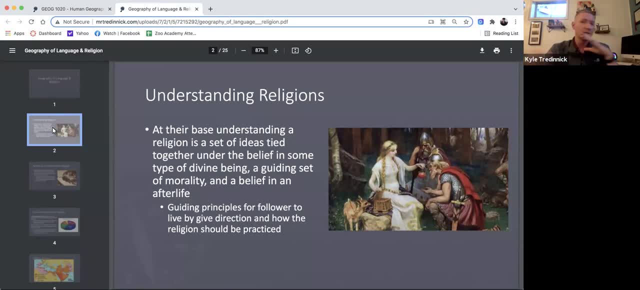 being or beings um that help dictate different factions or different um phenomenon, um. so i like to use the example of the norse or the greek or the roman gods here, because the gods had very clear, um very clear roles. where i'll use the example thor from norse mythology: um, he was the god of. 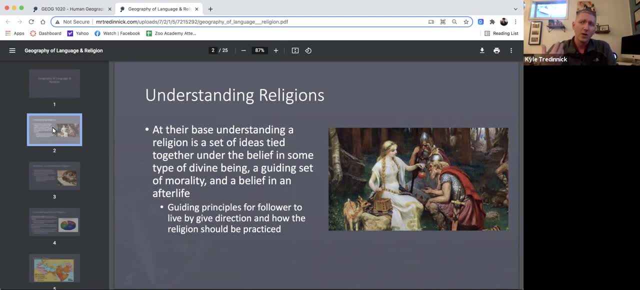 thunder and lightning and all that, and then there you had the god of tor tyr, that was the god of war, and then uh loki, who was the uh biotechnic on here, well, from if you're looking at the prose, um, so when i say prose, the prose, etta is one of the books that kind of 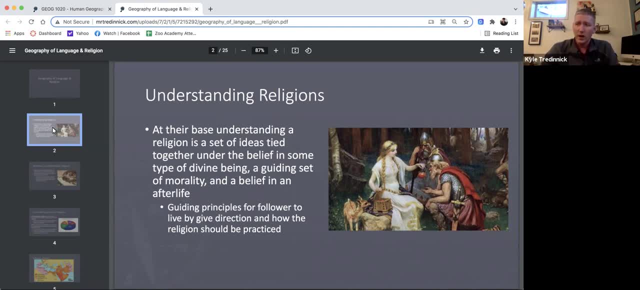 highlights different types of goddesses. um, so i think there's there's a lot of два conversation here. um, i think there's a lot of two there and i think there's a lot of three example. um, as well as ending all of the different sagas and all the different tales, um, going back to should have been snorri. 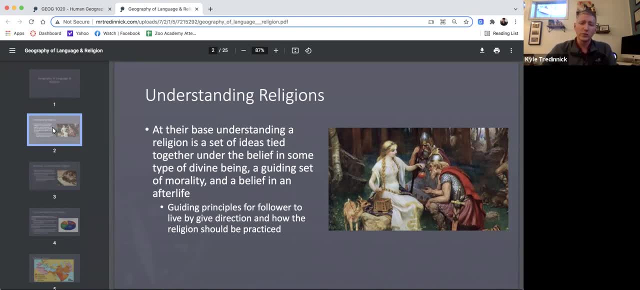 snorrelson, um, almost a thousand years now, or just over a thousand years now, that highlight this whole thing. but, um, yeah, in the prose and in the different books um that go along with norse mythology, loki was the? um god of mischief, but also, i guess, he's described as the doer of good. 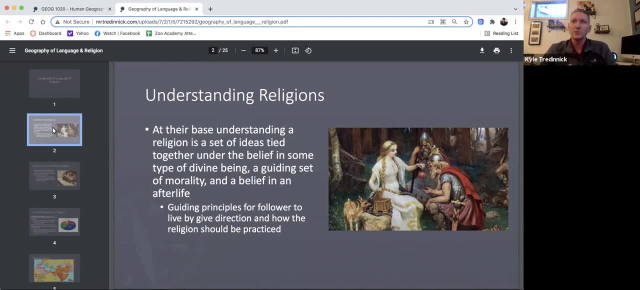 the doer of evil. so, um, it helps explain human behaviors. it gives the gods human behaviors and sometimes physical behaviors. so that's where thunder, we're trying to explain these natural phenomenon. it's a lot easier if there's some sort of divine being that is dictating how these um. 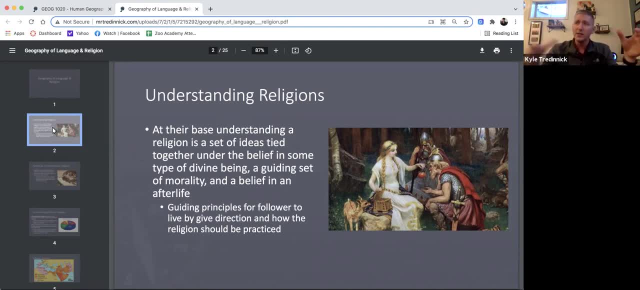 natural phenomenon are going. so, when trying to explain lightning and thunder, instead of understanding the rapid um um expansion of air based on the uh introduction of lightning and the heat that goes along with that, instead of trying to explain that scientific process or understanding that scientific process a lot of cultures resorted to: oh, that's the world, so this divine being that is doing it, instead of 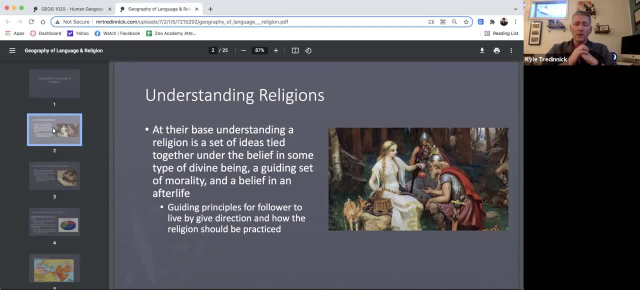 understanding the scientific process behind it. um, another thing that goes along with religions is a guiding set of morality: what's correct behavior, what's incorrect behavior, what's good, what's bad? um and then a set or a belief in the afterlife. this is where, um, the question comes up with, like buddhism, is: does it qualify as a religion? um, 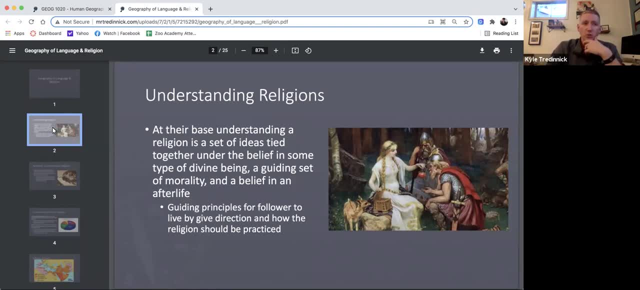 some, uh, religious scholars would say no, that buddhism doesn't count because it doesn't necessarily meet all three of these criteria. um, due to the process as or processes of reincarnation. um and so, since there is no belief in a necessary afterlife and the guiding principles of morality, 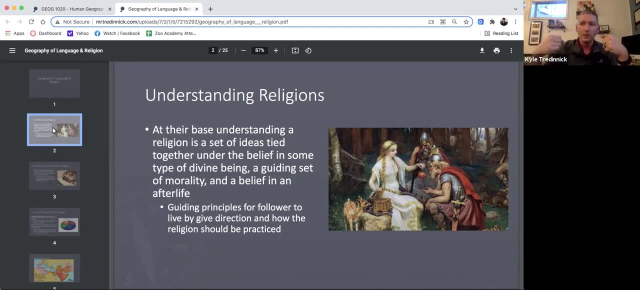 are really just leading to your next life. um, some religious scholars will not include that as a religious belief and we'll say instead, it's a philosophical belief. um, so that's where some of these distinctions get in. all right, and then the guiding principles is: just how should the religion 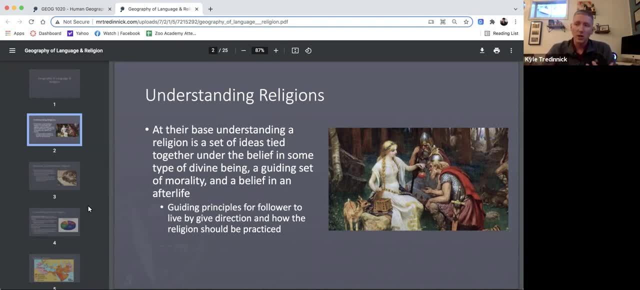 be followed and i'll tell you a little bit about that in a second. i'll tell you about the religion and i'll tell you a little bit about the religious tradition. um, i'll tell you about the religious. most religions um have some sort of guiding script or guiding uh book. so, like with christianity, 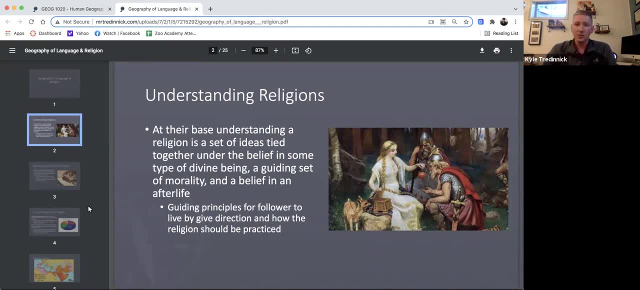 it's the bible, with islam it's the quran, with um judaism it's the torah. so, and then many, many, many religions will have these sorts of texts that lay out the principles of teaching its followers who is the divine creator, who is the divine or who is the divinity, um what? 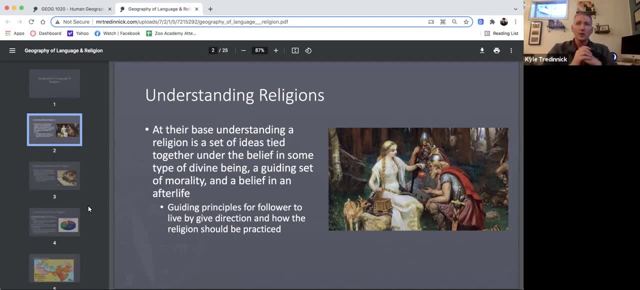 should followers of this religion do, and what is the outcome? um, is really what these books get into. um, some books are much older than others, so, like, uh, some religions were not codified as in written down because they were orally passed down and they were based on. 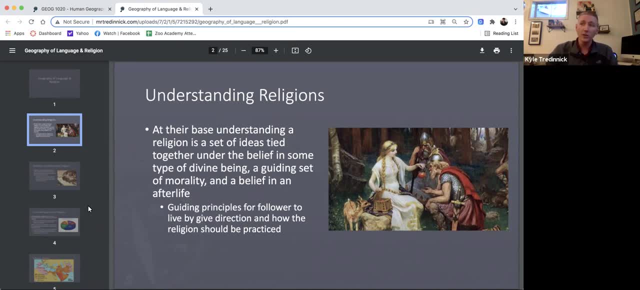 oral traditions. so, um, why i'm going into all of this is this is really helpful in us understanding the origins and then also how it spreads. so, um, a religion like christianity that is based on, uh, the book, the bible? um, it's based on literacy rates, so language and religion. 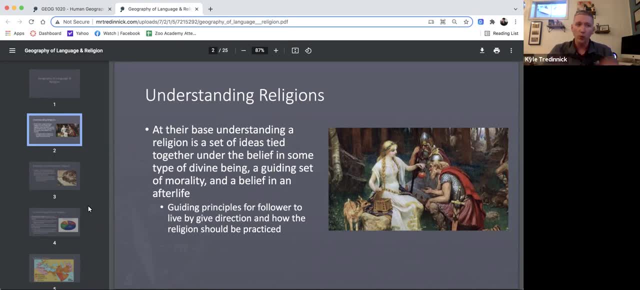 can very much be tied together. uh, same thing with the quran and its connection to um, um arabic. uh, and that's when we go back to the bible. there's the um division that goes on when the bible is exclusively in greek or aramaic or latin, versus when it's translated into german or 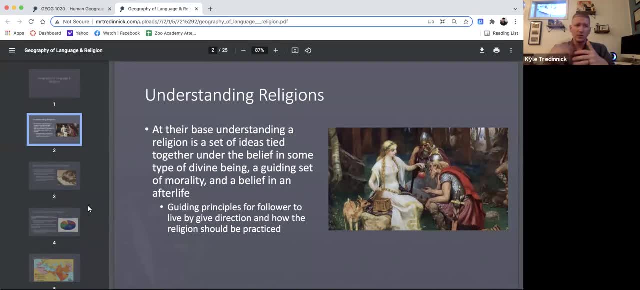 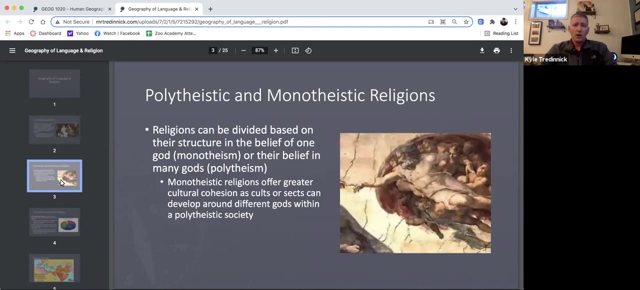 spanish or english or all those other languages, uh, that eventually come about as part of the religious reformations of 1500s or so. um, so, yeah, the connections of languages and religions are fairly close together, all right? um, i'm not going to spend too much time on this one, because this is one that 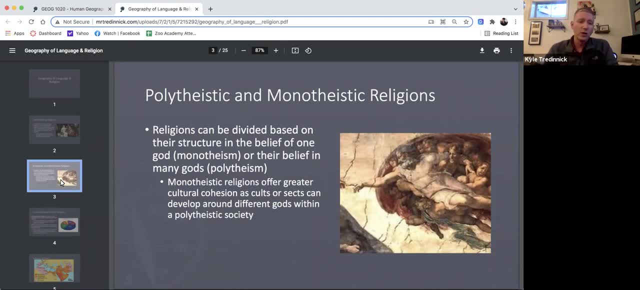 students usually get. but one way that we can distinguish between religions is money, or monotheism versus polytheism, uh, this just helps us understand and categorize different religions. so monotheistic belief in one main god versus, uh, polytheism, where it's multiple gods. 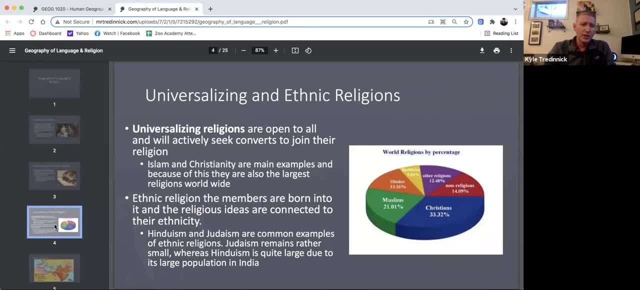 all right. another distinction that we can use in geography is the distinction between universalizing and ethnic religions. these will have a huge effect in the diffusion of these particular uh religious ideas. so universalizing religions, open to all um, so they will actively, often very actively, cert or seek to convert new members um through missionaries, through uh the spread of 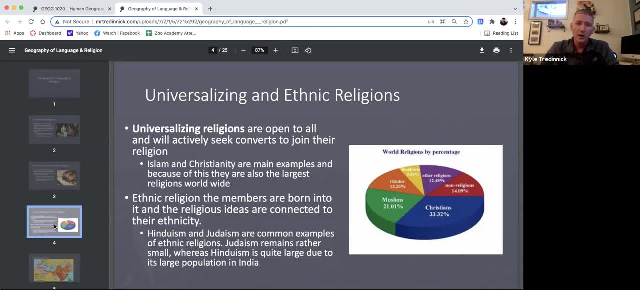 um, sometimes it can be political spread or military spread, um, but they will actively try and gain more members, whereas ethnic members the only way, or ethnic religions the only way that new members can join it is by being born into the religion. well, not, i shouldn't say only way, because 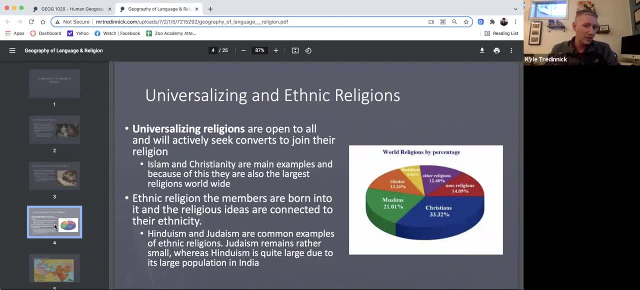 religions like, uh, judaism. there are ways to convert to judaism, um, but the main way that people join Judaism or Hinduism is by being born into it, Whereas Christianity, Islam, it's very much about the conversion process and the conscious decisions that go along with conversion, or acceptance of the faith. 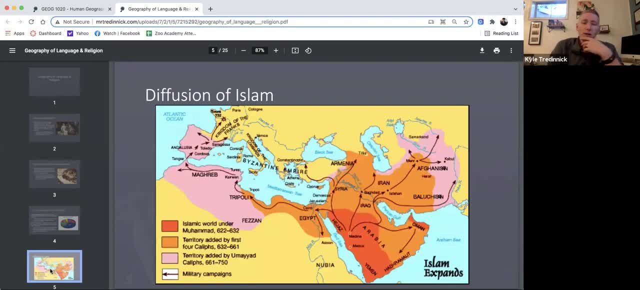 So when we're looking at an example here, looking at Islam as an example of a universalizing religion, that was very much tied to the argument could be said for political developments and the spread of different Muslim-based empires, but also, if you want to look into it some more, 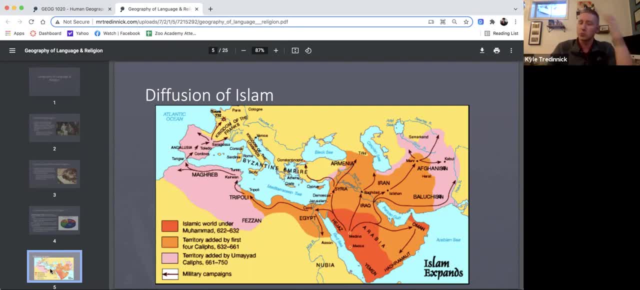 it's an economic spread, It's a cultural spread, where the Arabian Peninsula becomes one of the cultural hearths of the Middle Ages and many, many, many areas around Southwest Asia or the Middle East, North Africa. they converted not necessarily because of the political domination, but also because of the economic and the cultural denomination in that. 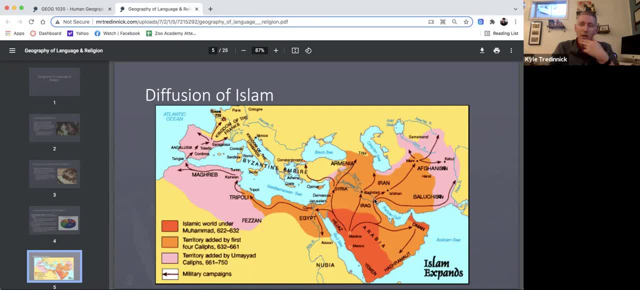 the Muslim empires that rise up and the Muslim empires that rise up. they become the economic powerhouses and you gain certain economic benefits towards being a Muslim. So a lot of people were enticed to convert to the religion for economic or cultural reasons, just because it was the big culture in the Middle East at that time. 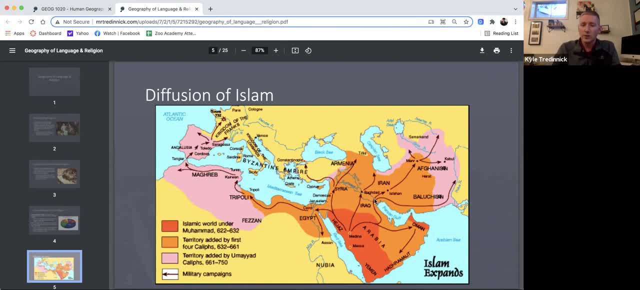 and continues to be the main culture or the main religious force in the Middle East, even through today. And yes, there are multiple religions that come out of the Middle East, but this is just one example And just looking that it was very much a. 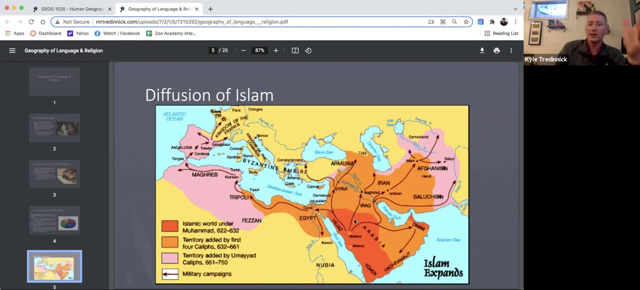 contagious diffusion where, starting out of Mecca and Medina and then spreading out the areas most closely connected to Mecca and Medina were the ones to convert first or for Islam to spread to predominantly first. So this is just a quick note. Islam is the religion, Muslims are the followers of that religion. 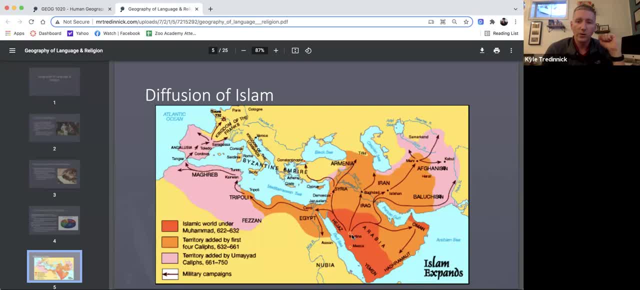 So, just in case needed to clarify that So, and then spreading out into the rest of the Arabian Peninsula, into the Fertile Crescent, into South Asia, Afghanistan, Iran, and then eventually on into more Central Asia, a region referred to as the Maghreb. 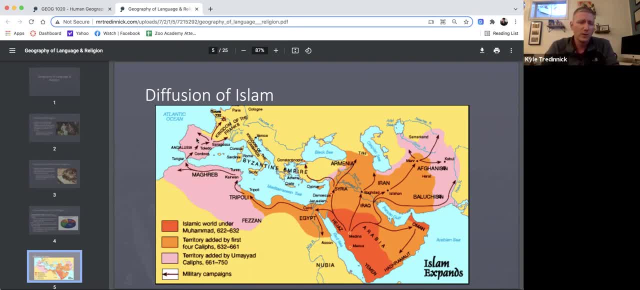 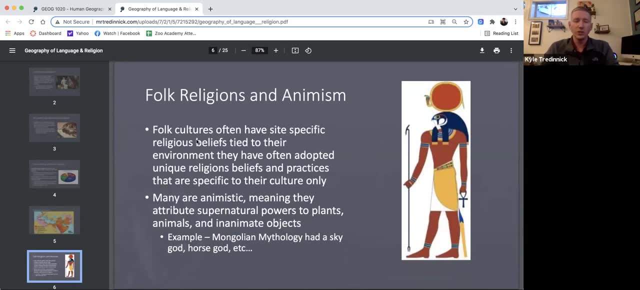 Northwest Africa, or literally the West, and then eventually on into Spain, So other religious affiliations or designations to look at. So folk religions, Oftentimes these are animistic, So animistic meaning. So the example that I've got here is the Egyptians. 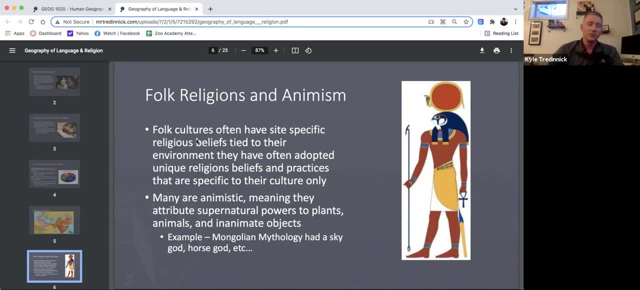 They've got the sun god that takes on, or you've got the different gods that take on different animalistic appearances, behaviors, and it's basically it's very much they're connecting their religious beliefs to their immediate surroundings, And so, with folk cultures, we definitely see this where. 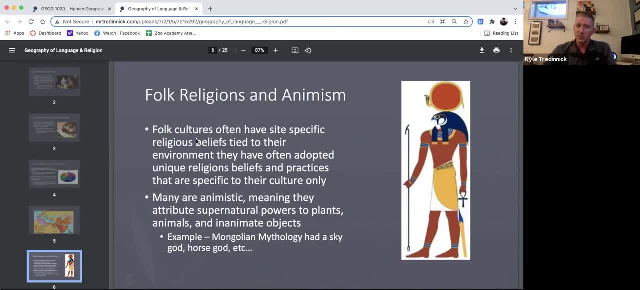 religion is more tied specifically to that location. So if you take the person from that location, you're taking them from, taking them from their cultural connection and their religious connection, And that was what was so wrenching for processes like the Indian Removal Act in the early 1800s. 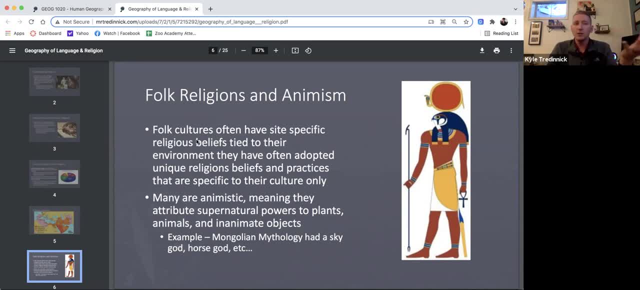 is removing American Indian tribes from eastern portions of the United States and moving them to the Great Plains or the American Southwest was, in essence, removing them from their cultural and religious homeland And their religion is so tied- or in many cases religion was so tied- to the landscape. 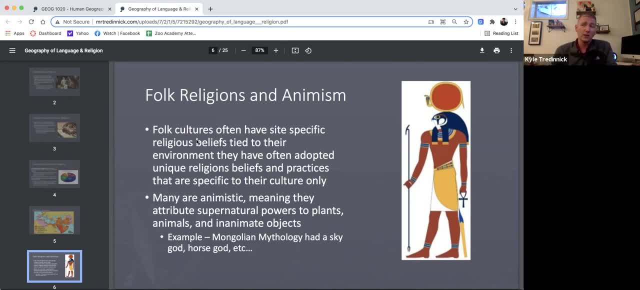 that it was effectively killing a lot of the religious connections by removing those people from their historical and that's why even today there's quite a bit of controversy surrounding areas all over the country because they still have religious cultural importance to people whose religions are tied to the land. 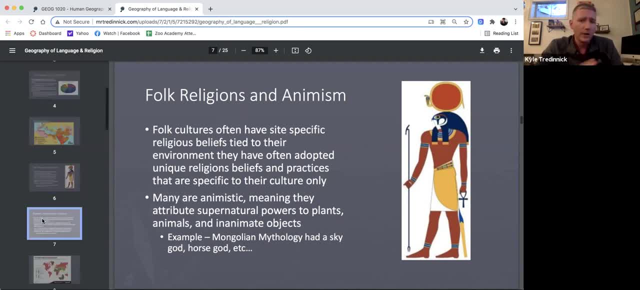 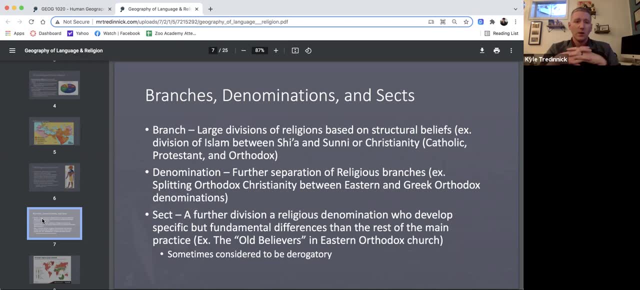 So there's that, All right. some other distinctions, So the distinction between branches, denominations and sects. So a branch- I'm using the very specific example here of getting all the way down to a specific sect of the Eastern Orthodox Church- 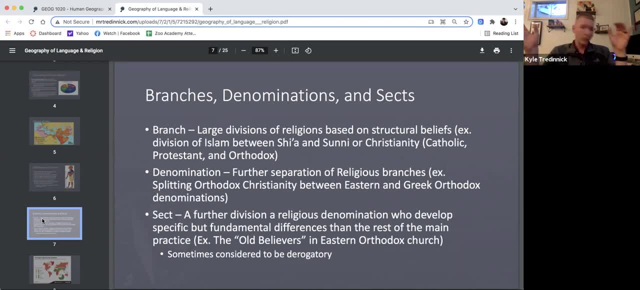 So to follow the path here using the different branches of Christianity. So Christianity is into Catholicism, Protestantism, Orthodox Christianity With Islam, Sunni Shia With Buddhism, again Buddhism, Even with the distinction Theravada, Mayahana, different distinctions there. 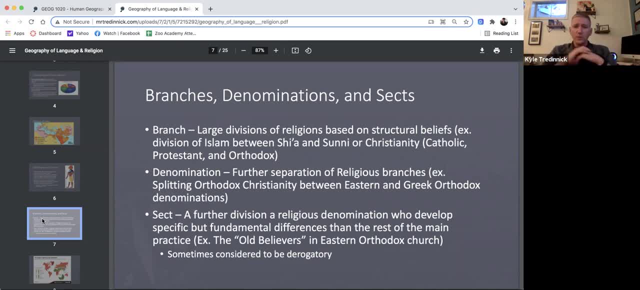 So, sticking with Christianity, though the specific branch of Christianity I'm going to look at is Orthodox Christianity, So very large, very encompassing branch of Christianity, down to the denominations. So the main denominations of Orthodox Christianity are: 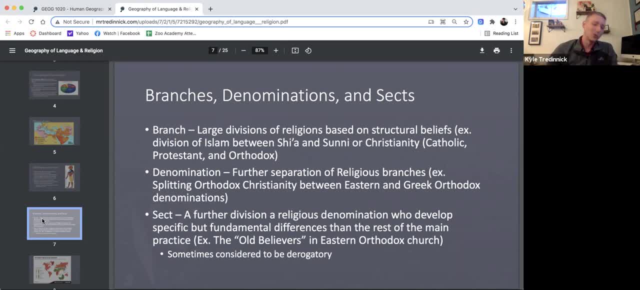 the Eastern Orthodox or the Russian Orthodox and the Greek Orthodox So very similar, and actually the Russian Orthodox can make the assumption, or the assertion, that it's actually Kiev, not Moscow, that is the center of this, Especially when it comes down to the diffusion. you could definitely make the argument that Eastern Orthodox Christianity belongs to the Ukraine. 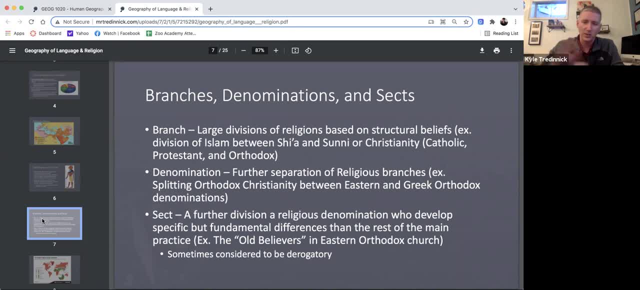 and not necessarily Russia, but the seat was in Russia for so long. that that's what we're going to go with. And then you could get down to the sects, S-E-C-T-S of these specific religions, where they're idiosyncratic or very minute differences. in the grand scheme of things, 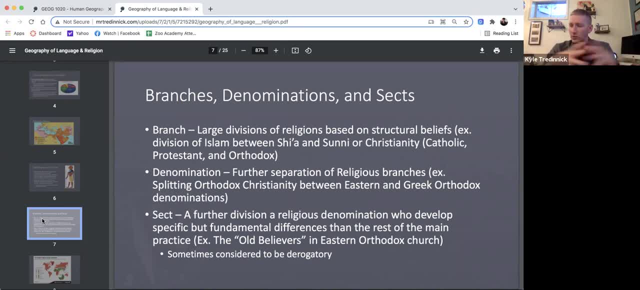 People within the different denominations or within the different sects. they might make the argument that there are huge differences. but so within these different sects, the example here is like the old believers in the Eastern Orthodox Church. Best way to explain them is: I don't want to make too concrete of conclusions here, but it's kind of like the Mennonites are to Protestantism. 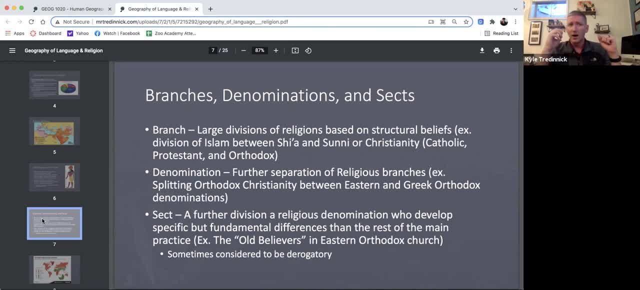 So more of a traditional way of belief, resistant to change, resistant to modernism and modern technologies. so the old believers actually ended up in like Siberia, to avoid the processes of industrialization, But that's just what their specific sect believed. 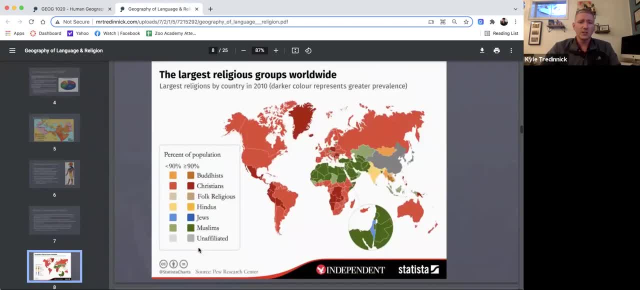 So there we go. All right, When we look at the distribution of religions around the world, we start coming up with some rather broad understandings of where religions take place. So Christianity throughout most of the Americas, well as the predominant religion throughout most of the Americas. 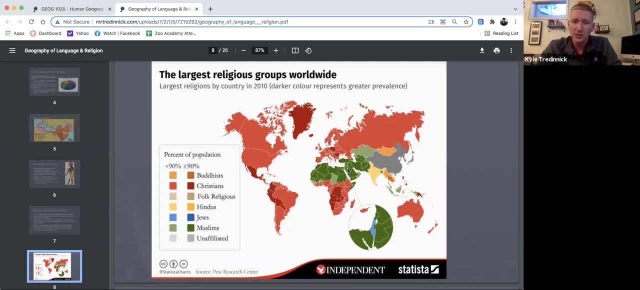 then Sub-Saharan Africa, and here we can still see the cultural influences and the remaining influences of Islam through Northern Africa into the Middle East and then into Central Asia and South Asia, and then Bangladesh and Indonesia, over here as well China as a decidedly non-religious state. 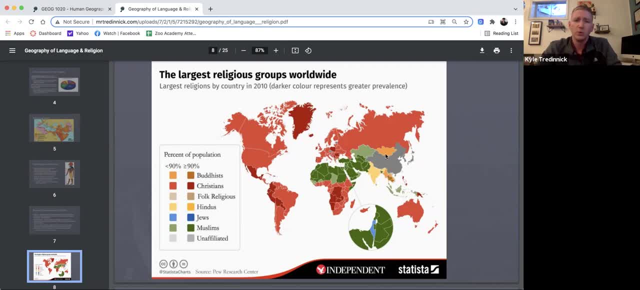 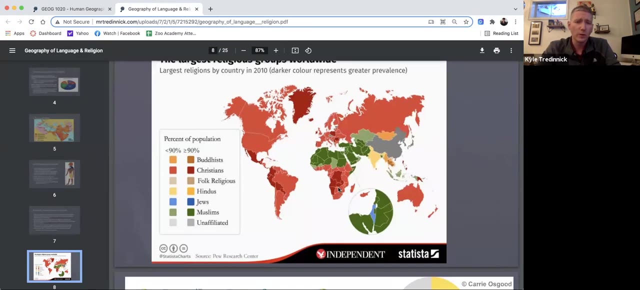 Hinduism and Buddhism in Southeast Asia and here in Central Asia as well, Judaism predominantly here in the modern state of Israel. So that's our wide distributions. but then when we break this down a little bit, we see another picture coming out of religion. 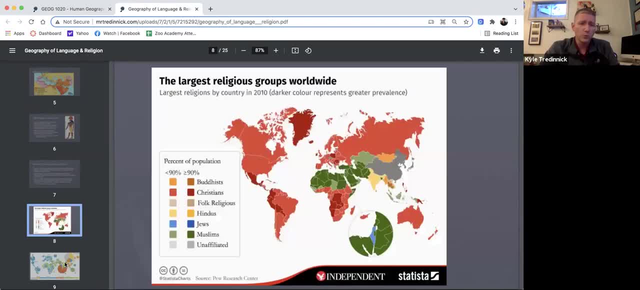 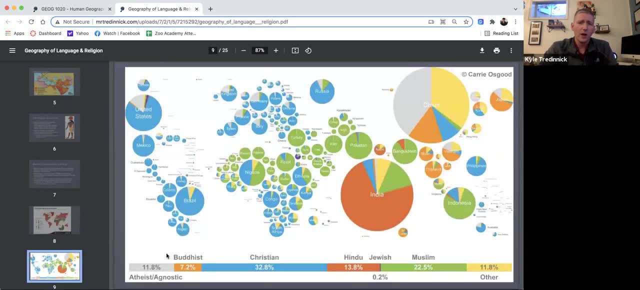 So we saw that United States was predominantly Christian and it's this little bit lighter color, So it's less than 90% And what we can see here is a little bit more complex understanding of how these religions are distributed. So we see that, yes, in the United States, quite a large majority of the country is affiliated with Christianity. 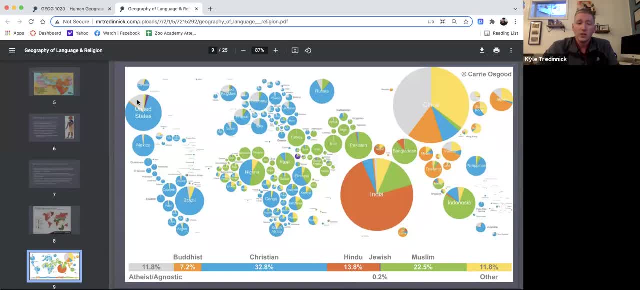 But then there's a large non-affiliated with Christianity, So a rather large chunk here. Same thing with Germany And actually unaffiliated. is one of the most rapidly growing religious denominations, if you can call it that is lack of religion. is one of the most rapidly growing denominations within Europe and North America. 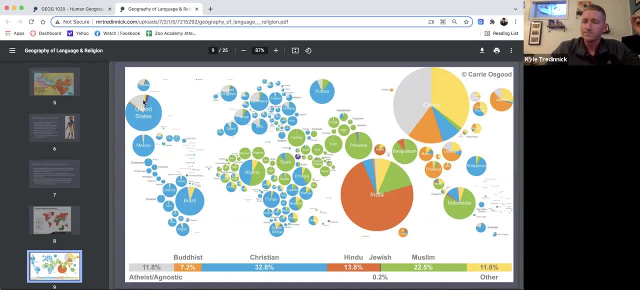 or what we would call Anglo-America, as in predominantly English, So United States and Canada, And that's just been tracked over demographics from year to year to year, And so here you can see that, yes, China has quite a bit of unaffiliated. 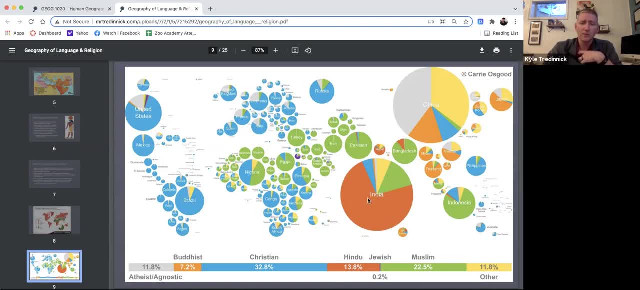 India is an interesting split where it's predominantly Hindu but then a large Muslim population, Then Buddhism as well- This yellow sliver. There's quite a lot of different religions. Sikhism and then Jainism as well are large religious denominations that you could find in India as well. 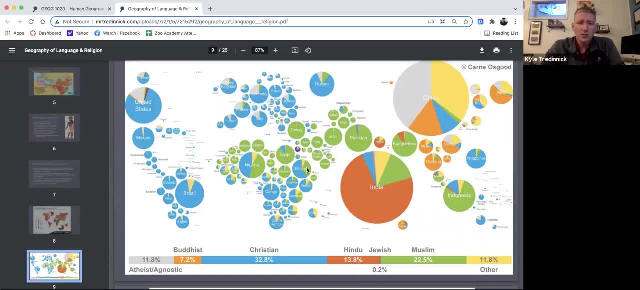 So why I want to show this is that this is an interesting look at, even where you've got countries where there's predominantly Islam, there's slivers or small portions of people of different religious faiths. So we can say that, yes, Nigeria, or yes, Egypt is a Muslim country and it's predominantly Muslim. 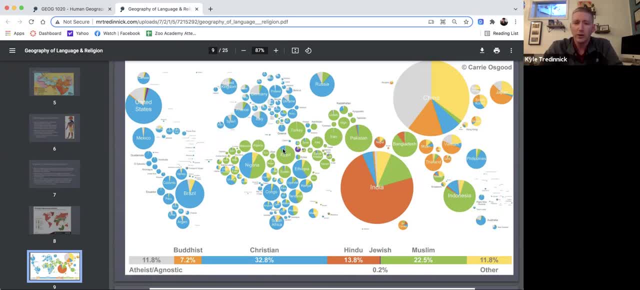 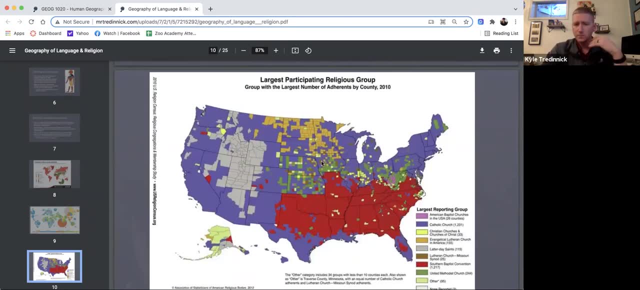 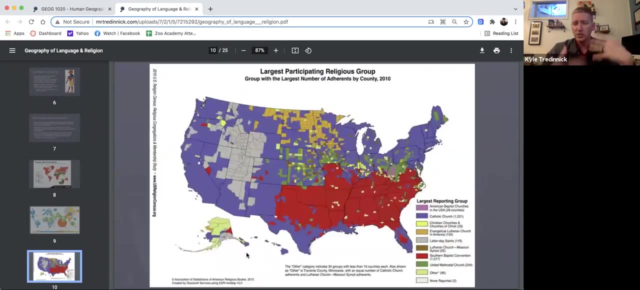 but then there's also a large Christian population here as well, And then if we look at, or look at this in even a smaller scale, we can start seeing some of these more denominations. So we go from international, So from international to more national scale, to more national and local. when we're looking at the division within the United States, 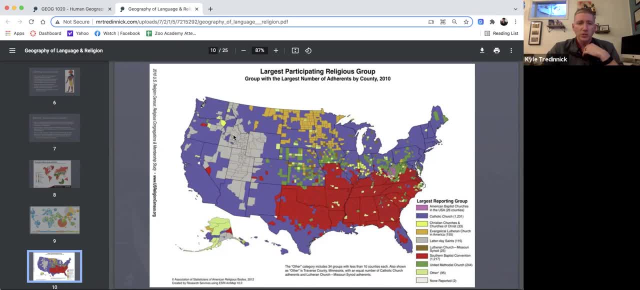 So you see large groupings of the Church of Jesus Christ, of Latter-day Saints, or as they're more frequently known, as is Mormons, but they prefer the Church of Jesus Christ with Latter-day Saints. Catholicism spread heavily through India. Catholicism spread heavily through India. 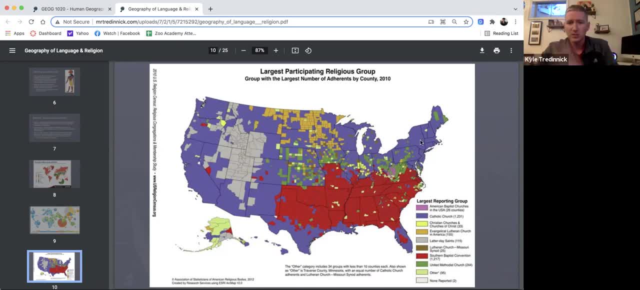 Catholicism spread heavily throughout the West into the Northeast. Catholicism spread heavily throughout the West into the Northeast. Evangelical Lutheran: connected to the spread of Swedes and Norwegians. Evangelical Lutheran: connected to the spread of Swedes and Norwegians. 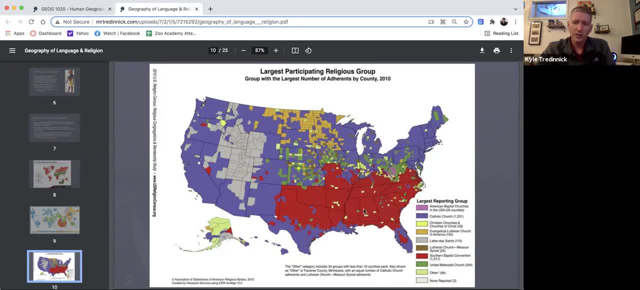 And then the Southern Baptist Church in the Southeast And then quite a few other churches all spread throughout, And so we see a lot of these, even county by county, And that's what it's looking at here is county by county. And so we're even still here. if we look at Lake of the Woods County in very northern Minnesota, here it shows up as evangelical Lutheran. 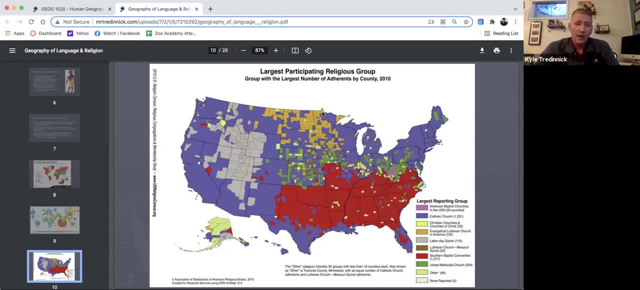 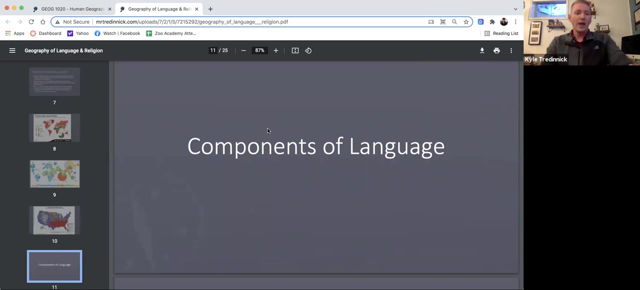 But that also means that there's most likely Catholics and other religious denominations here as well. it's just it's predominantly Lutheran, so we're only seeing the majority here. So limitation on this map, All right. Then when we look at language, 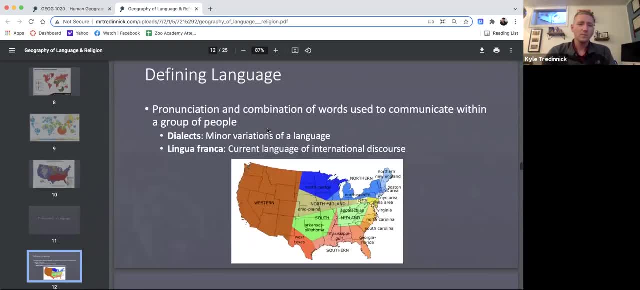 So we're just jumping right into this. one Language is a combination of words, pronunciations, and we can further divide them into dialects, so these are minor variations, And this could be British or UK English versus Irish English, versus Scottish English versus Eastern United States English, and you can get into all these different dialects. 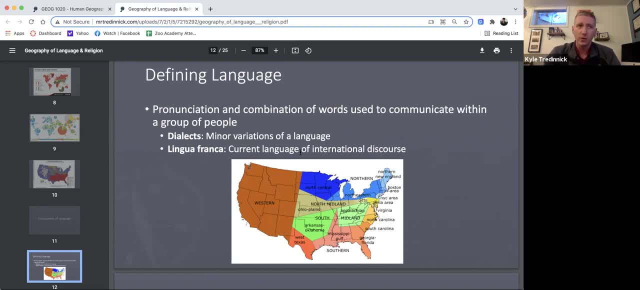 And then when we, And then when we, And then when we, When we go into the next segment, We're going to look at slang And the first distinction we see, or another important distinguish meant, is this: lingua franca. So right now, and actually for quite a while, 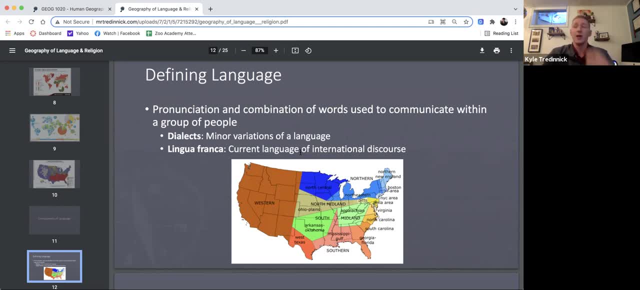 The lingua franca for the world has been English, and it's not necessarily because of the dominance of the United States, but it's we kind of inherited the dominance of the British empire, where people learn to speak English so that they could continue to speak English. 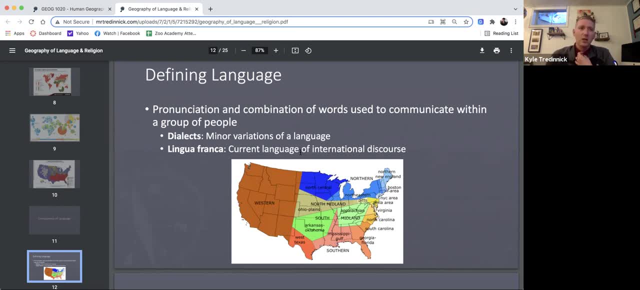 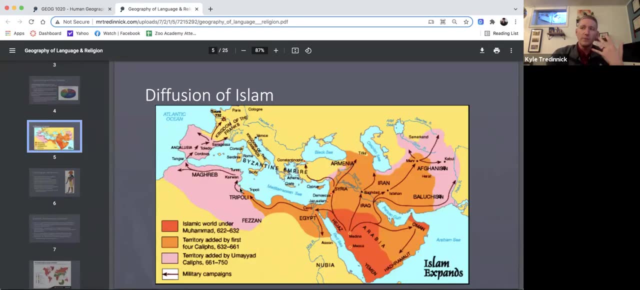 English that they could continue to do business with this large economic power, which- that's one thing that I was trying to describe here, too- is that people learned Arabic and converted to Christian- or not Christianity- Islam, so that they could take advantage of the benefits of being affiliated. 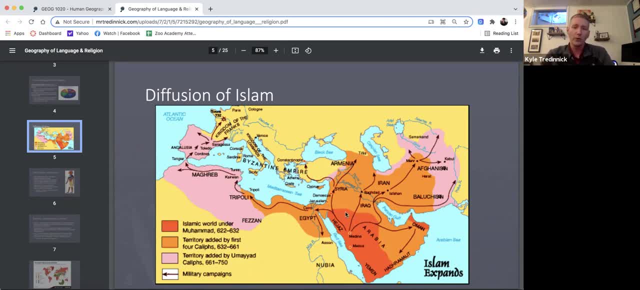 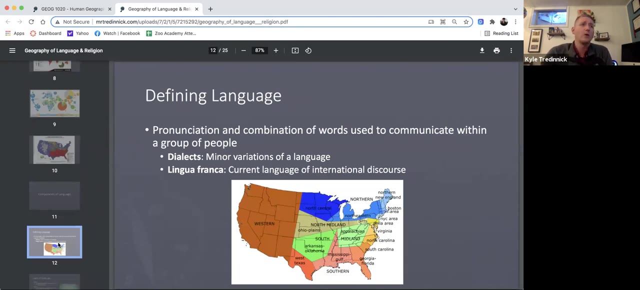 with the large economic and cultural power in this area And then not to diminish them and say that it wasn't for personal reasons as well, but when we're getting down here into the lingua franca idea, is right now one of the largest English-speaking countries in the world and I believe it is the 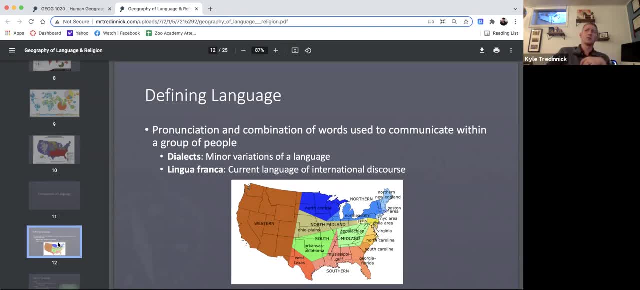 largest is India, And it's just because that's still one of the. in a country that has so many different languages and so many different religious denominations and so many connections with other countries, it's just easiest to learn English to be able to do that, And another good example is actually: 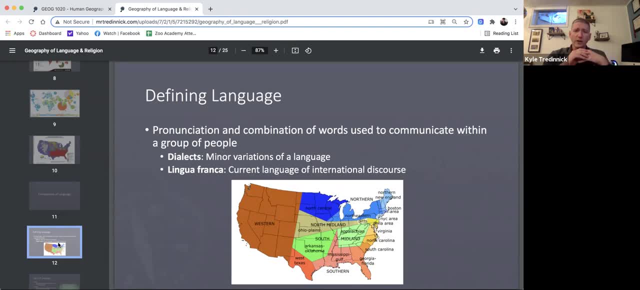 Iceland, where Iceland the lingua franca. like everyone speaks Icelandic, but then also everyone speaks English. So if you ever get the chance to go to Iceland as an American, it's incredibly easy. just because everyone already speaks English, even older populations, And it's because, long ago, 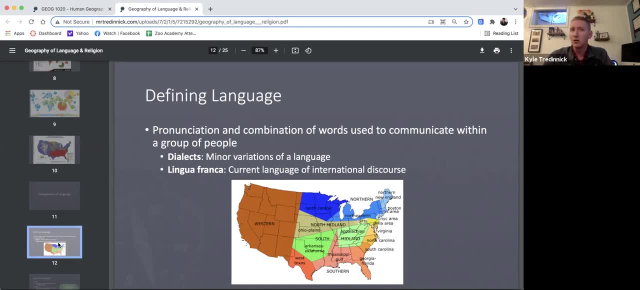 they understood that it was a language that they could learn, And so I think that's one of the things that's really interesting about this is that it was much easier to just teach everybody English than it was to try and translate all their books into Icelandic. And so in schools, 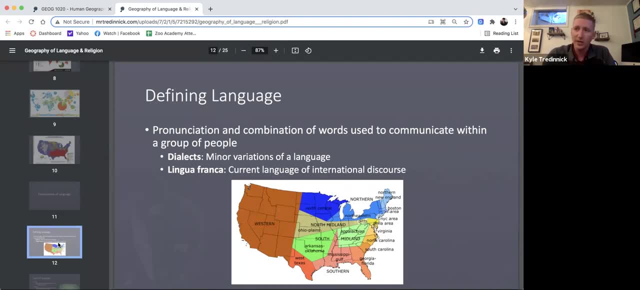 instead of trying to translate every single textbook or every single book that they wanted to use in classes, they just had their students learn English, just because it was such a powerful language for them to learn, And it's helped them with their connections now with their tourism. 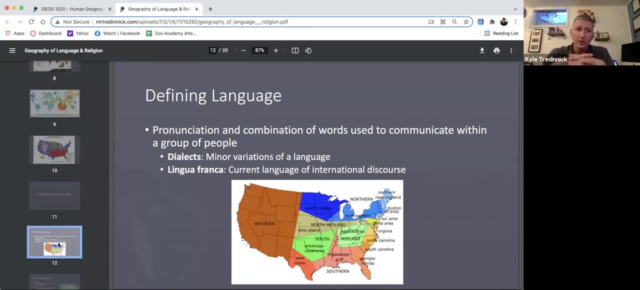 industry. Tourism is another one. Yeah, So there's one other question I have is, especially when you're teaching your students, where, if you have a little bit of English that you think makes them feel like they've been taught Maersk. 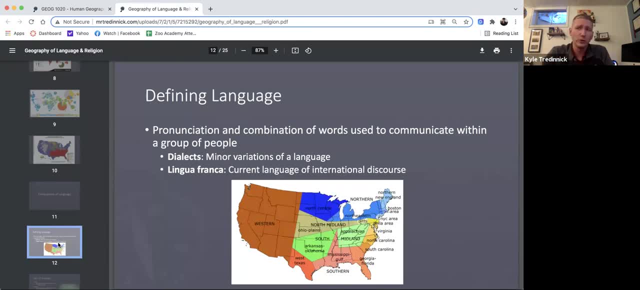 I think the second question there is: as long as you speak English, you're kind of set just about anywhere you go. With all the countries I've been to, very few did not speak English. Actually, the country that I would say was the least, the least already connected with being able. 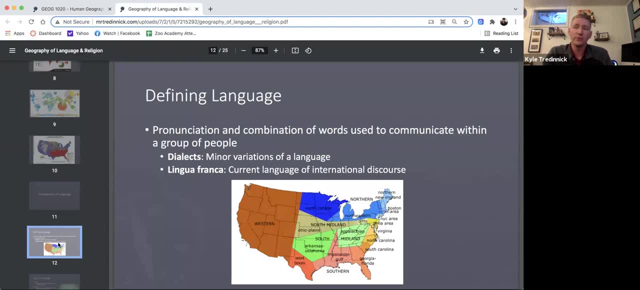 to speak English, would probably be Russia. So Russia, Yeah Right, I like that name. Yeah, Yeah, Yeah, Yeah. Yeah, very few people spoke English there compared to other places that I've been, So and that's because Russia has- or, yeah, Russia has- established Russian as the lingua. 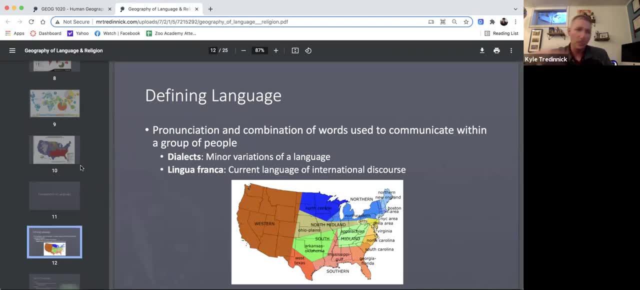 franca in Central Asia and Eastern Europe, to the point that they define themselves as a, or they have arranged themselves as the dominant cultural influence, to the point that why would people learn English if most of the business is within their sphere, And so that's Russian? 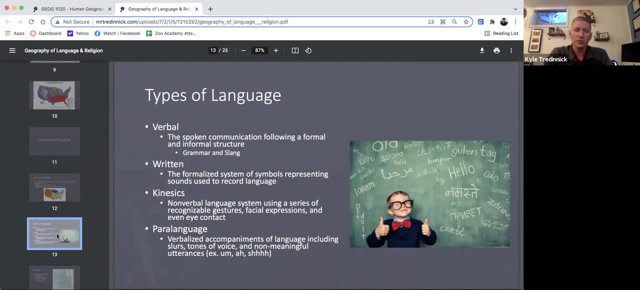 So the types of linguistic or the types of language communication, So you can get into the verbal and the different ways that people speak, The written languages, which that's pretty self-explanatory. The kinesthetic or the kinesic is the. 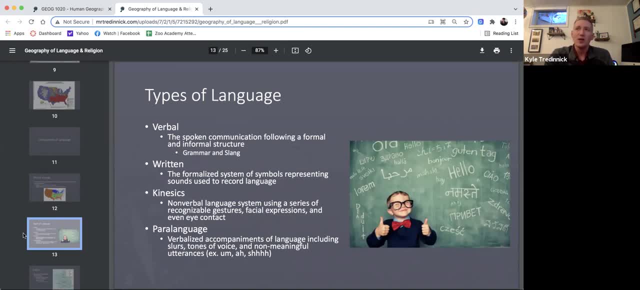 The motions. A lot of people would point out the hand gestures in Italian, and it's a very animated language with a lot of hand gestures- And then the paralanguage. These are the ums and the ahs and the kind of words, but not really words that are included. 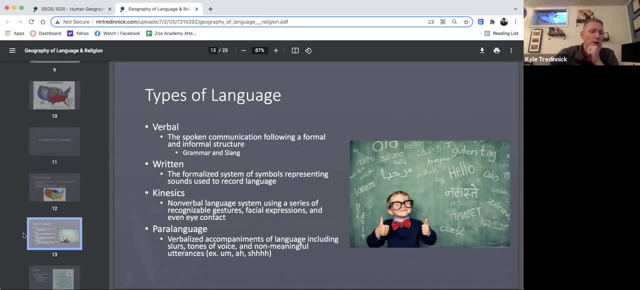 with language And this can get into slurs, This can get into idioms, Idioms I was looking, I was looking at just the other day there was a map that was looking at the idioms, or the idiom equivalent to. it's all Greek to me. 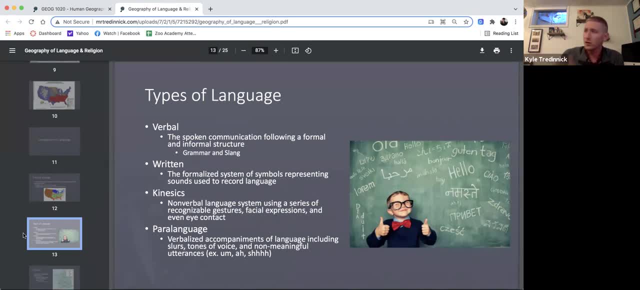 The way to say that if I were to look at another language, I don't understand it. It's all Greek to me And it was a map of Europe and it was looking at like Eastern Europe. the similar expression was: it might be Greek to me. 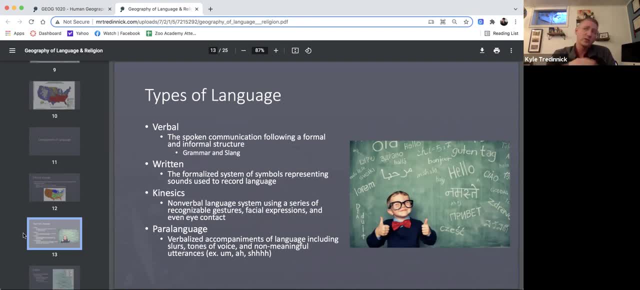 It was, it might as well be Chinese and Western Europe. It was, it might as well be Spanish. And then the one that I thought was funny is the most direct connection, or the most direct equivalent to the phrase. it's all Greek to me in German, the it roughly translates: 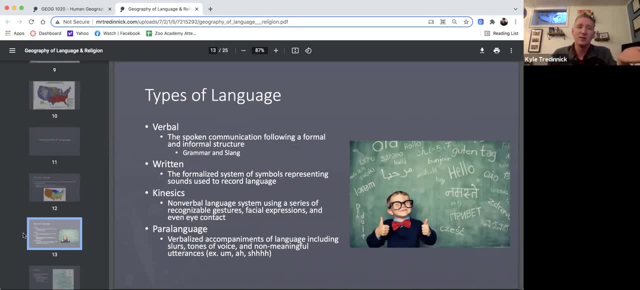 into I only know train station, which I thought was kind of funny because that was one of the pieces of travel. That was the first piece of travel advice that I got early on was that whenever you go to a country, learn how to say where is the train station. 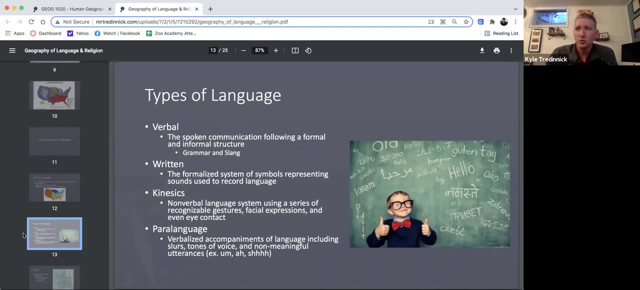 Because that way the person you're talking to will know that you're a foreigner, in case there was confusion, And the train station always had someone who would be able to help direct you to where you needed to go. So I think that that's funny that that's still reflected in this idiom in the Germanic language. 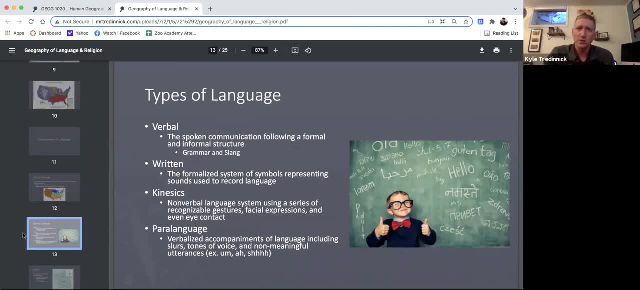 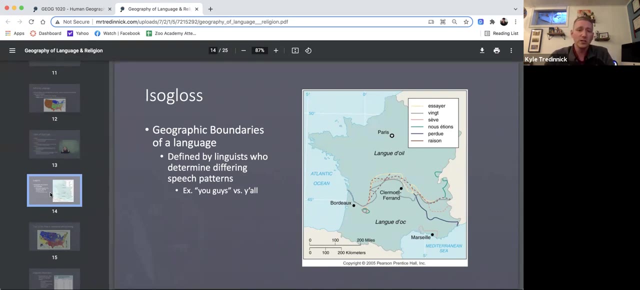 or in the German language, That instead of it's all Greek. to me, the expression is: I only know train station, So that's where all that comes from. All right, A very specific geographic term connected to the study of language is this concept of. 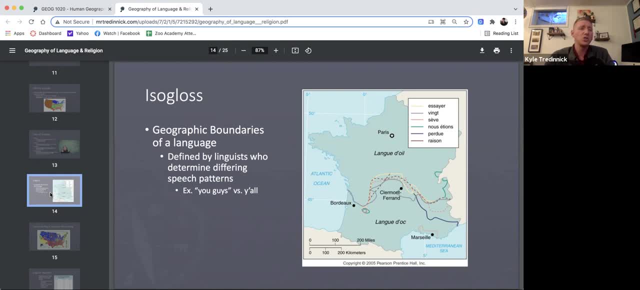 an isogloss. So this is a geographic boundary in language. A very clear isogloss that I can think of, or that I would bring up here, is the division between North and South, North Korean Korean and South Korean Korean. 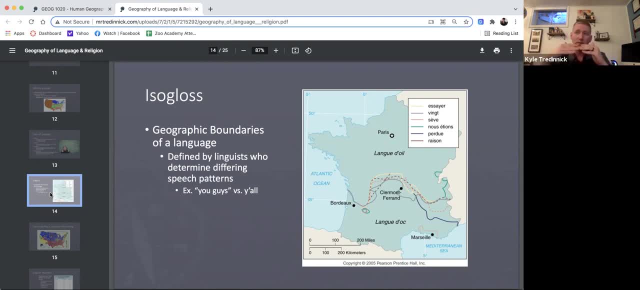 And it's very distinct along the DMZ or the demilitarized zone along the 38th parallel And because this division there hasn't been really any cultural connection across the DMZ or this border to the point that North Korean has almost kind of evolved as its own. 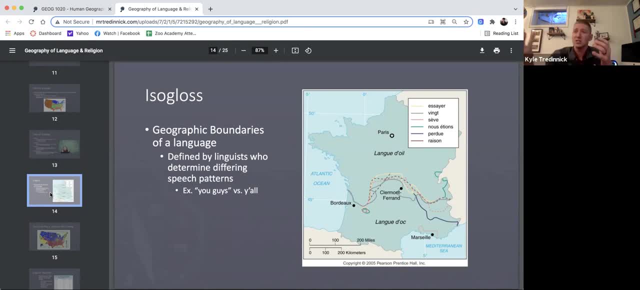 separate form of Korean. There's words that just simply don't exist in North Korean, that exist in South, Just because South Korea has so many more cultural connections and they have access to groups and technologies that just are not available in North Korea, to the point that 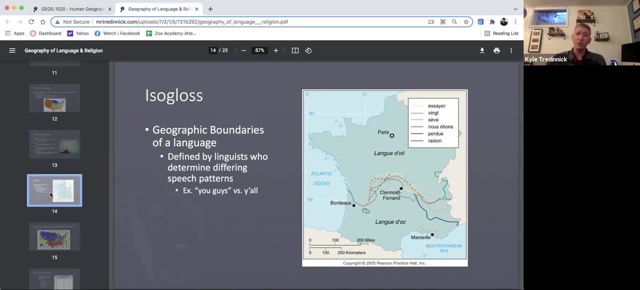 there's the question of whether or not to classify them as two different languages anymore, And it's just such a stark division at the border, Whereas some of the borders can get a little bit more muddily. where you're looking at, say, the French region of Alsace-Lorraine kind of over here, where, yes, it's within. 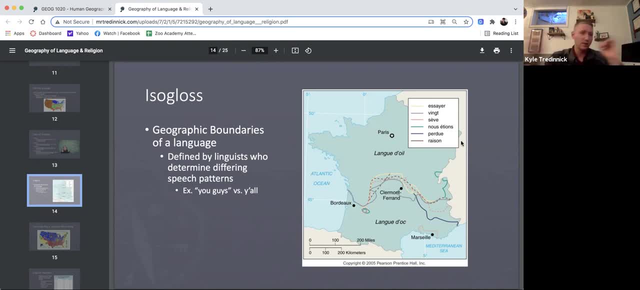 France, but there's been a- let's call it- a conflicting history where sometimes it's part of Germany, sometimes it's its own thing, And so it's got a lot of cultural heritage from all of these groups, And so it's not as stark or as well-defined of an isogloss. 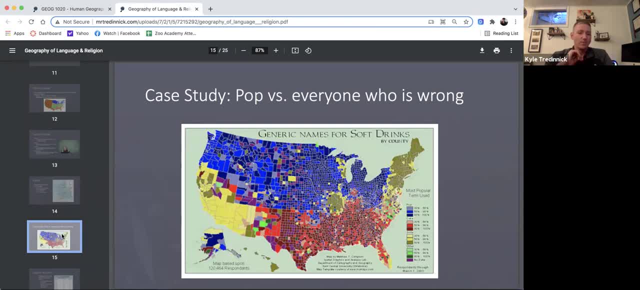 So an example of isogloss Is the study of what people call a carbonated beverage. So I titled this as pop versus everyone who's wrong, because pop is, I mean, very few things you can be wrong in here, but if you're not saying pop, you're wrong. 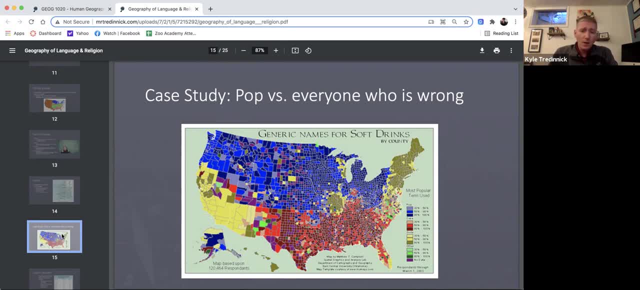 So that's just how it's going to be. But who calls it what? So when you get into central Missouri, suddenly it's soda. Wisconsin it's soda, but then most of the upper Midwest it's pop. And then you get down to the South and the Southeast and you're getting into Coke. 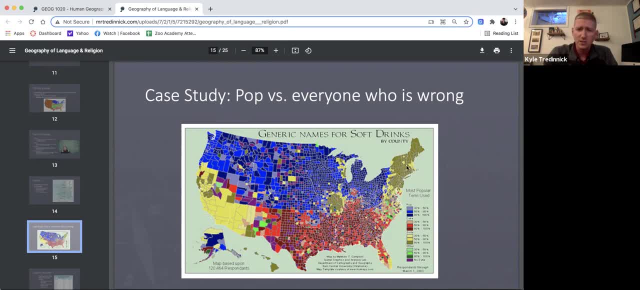 And then suddenly you're back into soda land. Northeast. it's kind of this mixture of many different things, but we've got soda predominantly, And then down here in the Southwest again soda. So yeah, it's this mixture And then other it's. yeah, they're kind of all over the place in what it can actually. 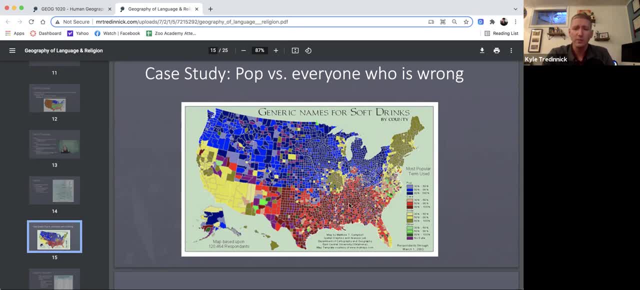 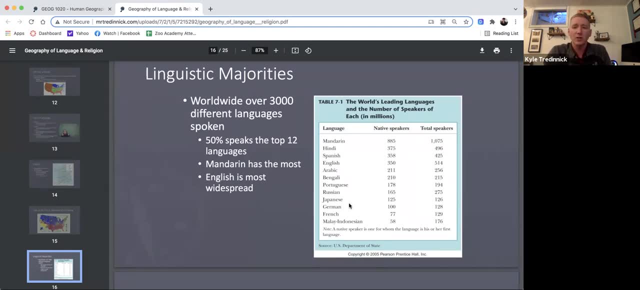 be defined as Soda pop is one of the others that comes up every once in a while. So when we look at linguistic majorities on a international scale, what we see is that most people, so about 50% of the people on the planet, are in one of these 12 languages. 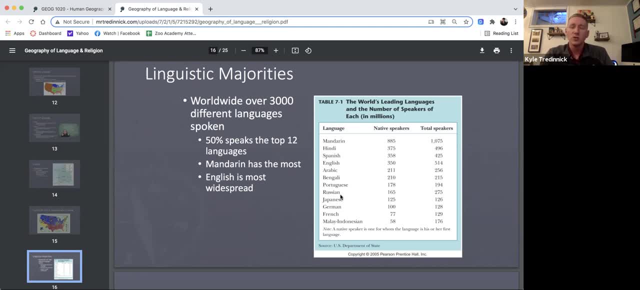 with Spanish Or not Spanish, with Chinese Mandarin being the top Hindi, second Spanish. then we get to English. So, and this is native speakers. So, when we look at native speakers, yes, Mandarin Chinese is one of the largest native speakers. 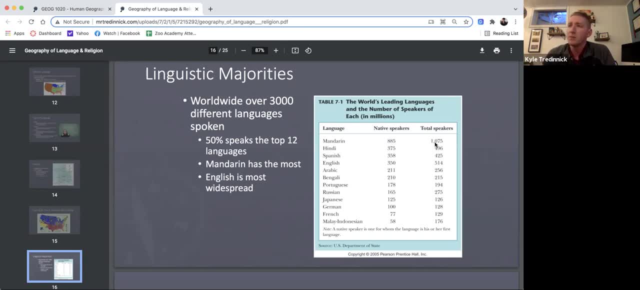 but then there's a lot of people who don't speak Mandarin Chinese as their primary language. But then, because Mandarin Chinese is the Linguafranca for China itself, everyone within the country, regardless of whether or not they're Han Chinese, which Han Chinese, are the main speakers of Mandarin Chinese. 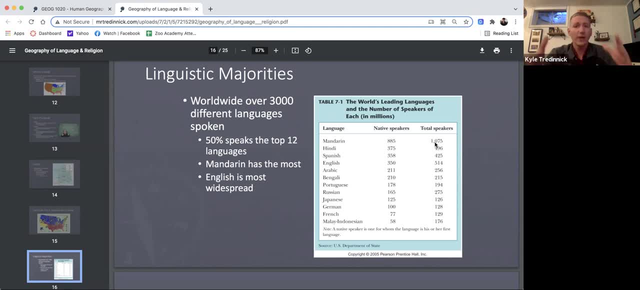 as native speakers. Everyone has to learn Han Chinese or Mandarin Chinese. even if they're predominantly Cantonese speakers or from Cantonese regions of China, they also have to learn Mandarin. And then we actually see that for this, English Is the second largest for the total speakers and that reflects English as the Linguafranca. 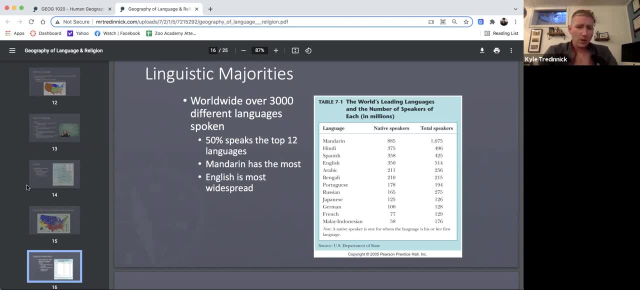 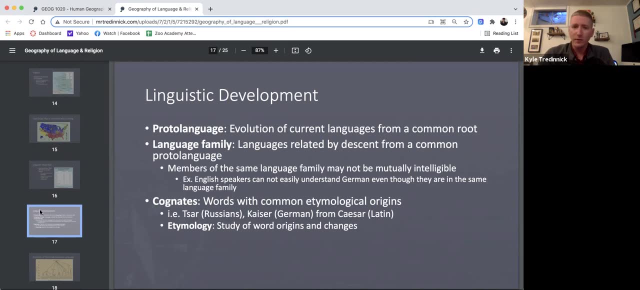 internationally. So, all right, The proto languages is just the evolution of a language. Language families is the descent from a common proto language. So English is a Germanic language family or coming from the Germanic language family, Whereas French is coming from the Latin language family. 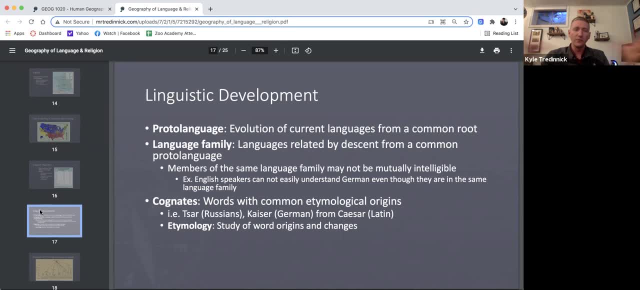 So at one point the language is kind of evolved from that one language hearth and then cognates, especially more recently or as languages have had more connections with one another. you see a lot more cognates where instead of developing or instead of having words unique, 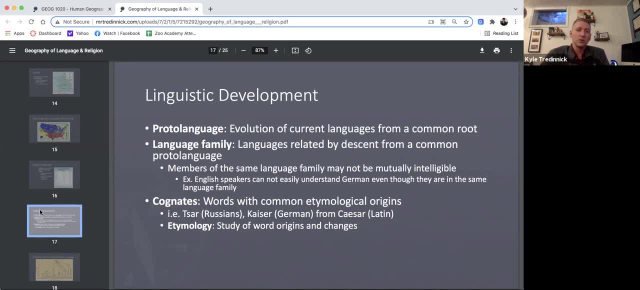 to that language. they'll use languages or they'll use words, Words from other languages. So the example that I've got here is czar is the Russian word for Caesar, or Emperor. Kaiser is the German word for Emperor, And then Caesar is the Latin word for Emperor. 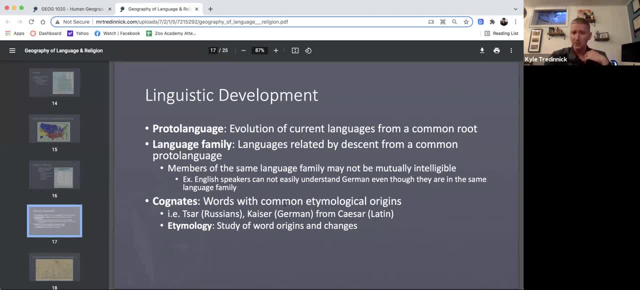 So czar, Kaiser Caesar, sound very similar to one another, but three very different languages and from different language families. And this etymology is the study of words, their origins and their origins And their changes throughout time, And so it's still a linguistic track of trying to understand where did words come from? 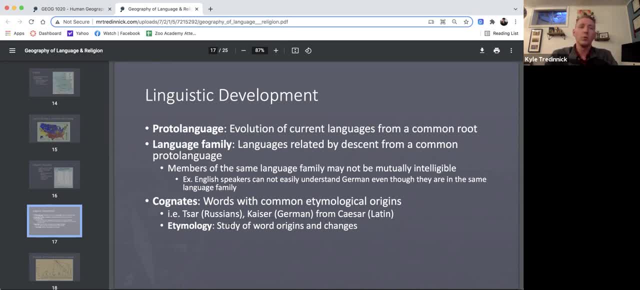 How did language develop? And so with English especially, it's complicated because it's got so many connections to different Germanic languages. So Anglo-Saxon is where English comes from. So it's complicated. So Anglo-Saxon is where English kind of derives from, but then it's got the Welsh connections. 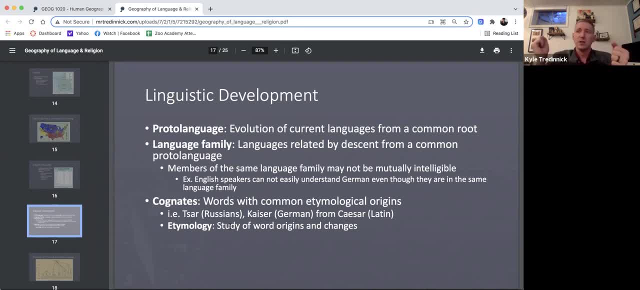 It's got the Britain connections, because that's really where English develops is on the island of Great Britain or on the islands of Great Britain, And there's Welsh and Cornish and Scottish and Gaelic and all of these contributing, or in the area contributing, to the development of English. 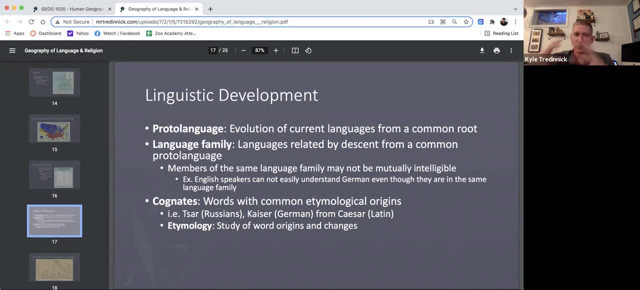 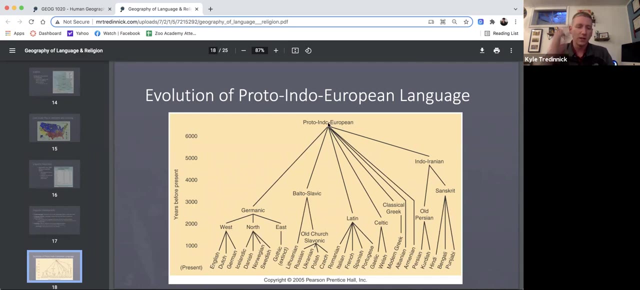 And then there's English as a language, but using the Anglo-Saxon language as a root- German root- that is then built upon and evolves to become English as we know it now. So if we look at the example, the Indo-European languages, a common root. from that comes the. 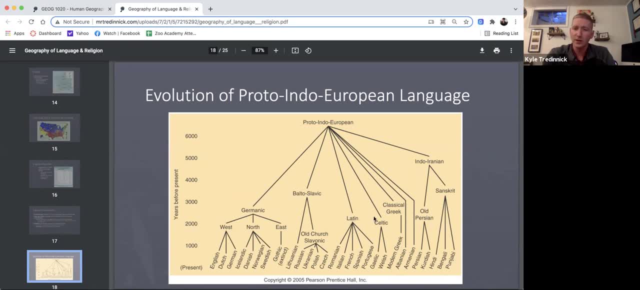 Germanic languages, the Baltoslavic, the Latin languages, Celtic, Greek, Persian or the Iranian Indo-European languages, So Indo-Iranian, which includes Persian, into all of these different languages they derive from the same place. And how we know that is just in the development itself and a lot of it is the etymology which 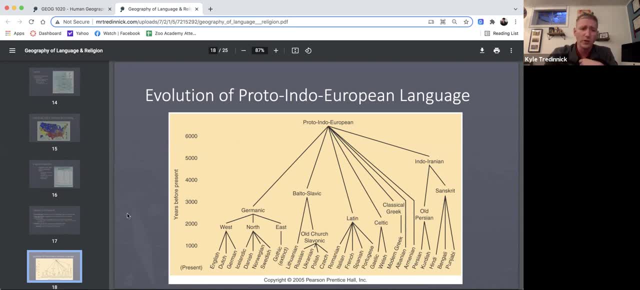 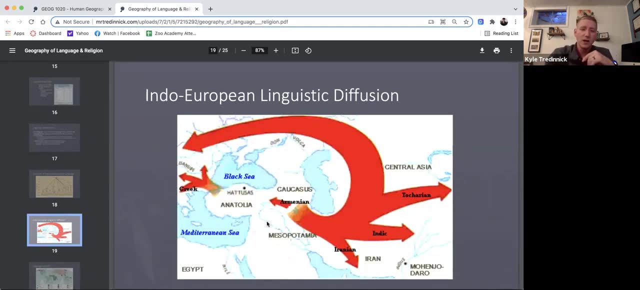 almost kind of like the genetic code of each language And we can look and start surmising and theorizing how this develops. is a common root from the Caucasus, from which Iranian eventually splits off. Latin becomes its own language, family Indian or Indic splits off. 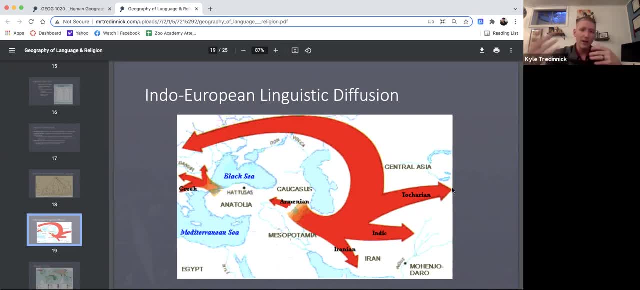 What eventually becomes the group that will develop Mandarin, splits off, And then this group swinging around will be the European branches of language, whereas got another branch coming out of Turkey, And so we just look at a lot of the similarities and a lot of the connections. 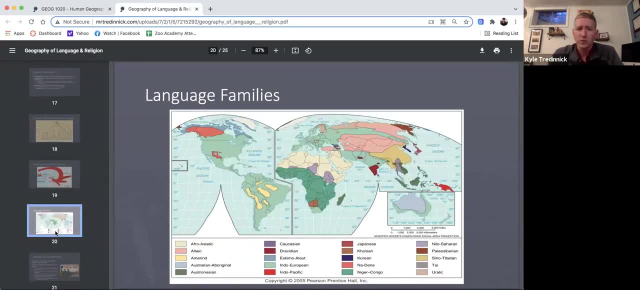 And what this leads to is a fairly unique or fairly diverse language separation where we've got still in the Americas. so the American Indian languages or the more So the Paleo-Siberian is the connection to old indigenous groups from Siberia. Okay, 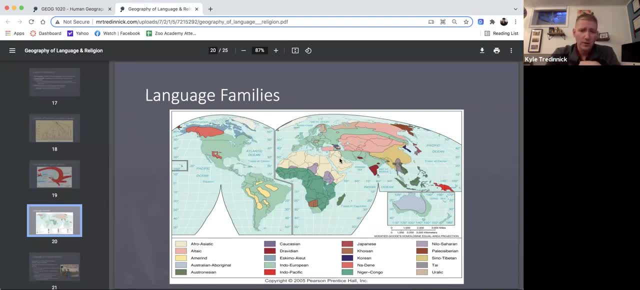 But if we look at the spread here, so the Arabian languages very much connected to the Arabian Peninsula here, then the Niger-Congo language family, the Indo-European. What I think is really unique here is we see the main connections with Finnish a little. 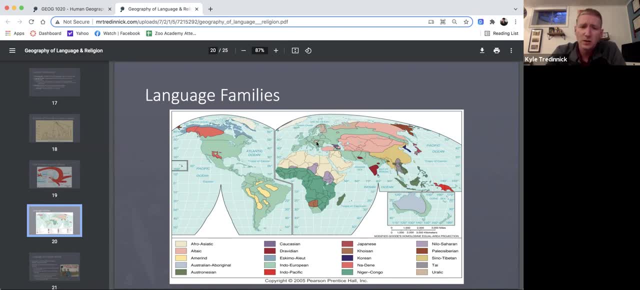 bit different: the Sami region of Sweden, Slovakia, its own thing. But then when we look at Russia we can really see the impact of cultural diffusion is connected to the spread of technology, because this almost perfectly follows the path of the Trans-Siberian. 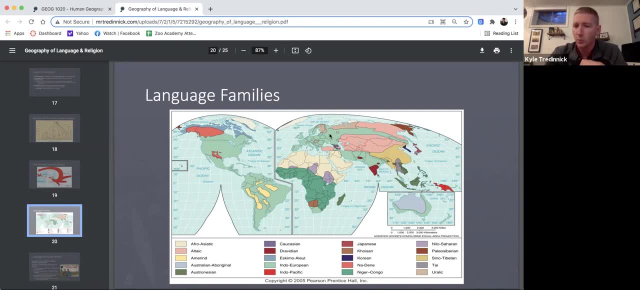 Railroad And so we can see that where the Trans-Siberian Railroad went really heavy influence of Russian language into the Far East. that kind of splits the Altaic religion and Not religion Language in half, Just because along here it goes again into economic political power of the Russians. 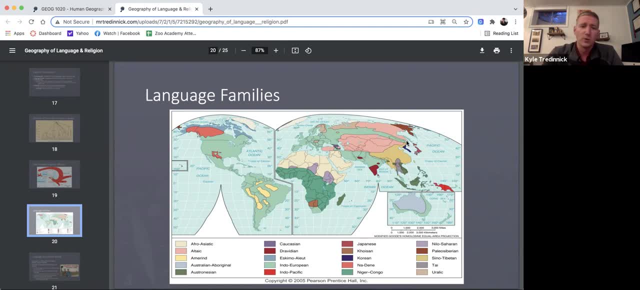 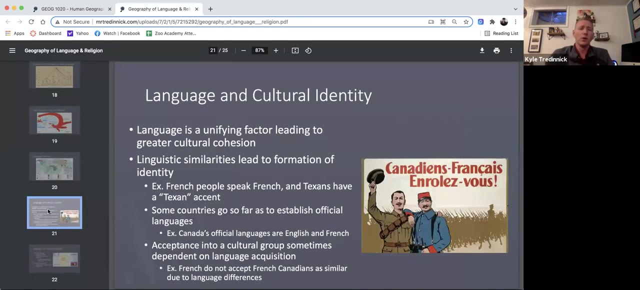 that spread along this railroad route that went east all the way from well Moscow. Moscow is the center for the Trans-Siberian. It's really confusing, but that's how they developed So language, why language is so important to all this. 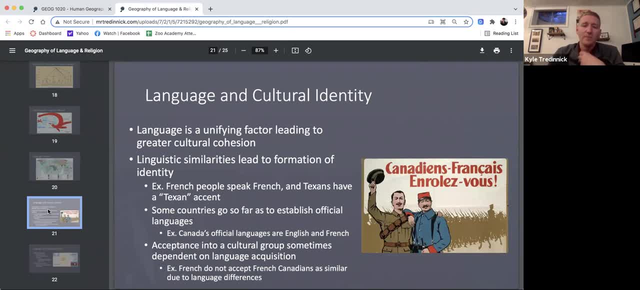 Because it really helps understand the cultural identity. So I like this World War I recruitment poster where it's French Canadians join the army is essentially what it's saying: or enroll or sign up, or you should sign up, And it was connecting to the French Canadian, or it's trying to build the French Canadians. 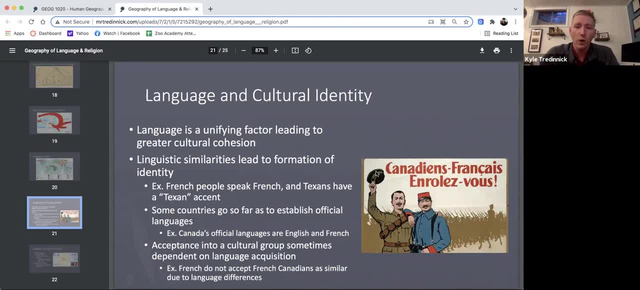 to the French in World War I and saying: hey, French Canadians, you're very much connected to the French, You share the same cultural identity, So let's go help them. And so that's really what this is showing, and it's appealing to their cultural senses. 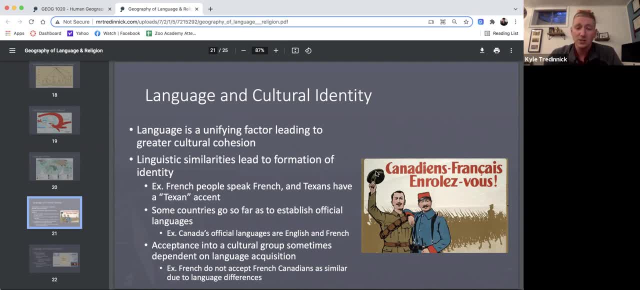 and their cultural identities to the point that saying, hey, yes, let's go get involved in World War, I Go help out your common linguistic brothers, And it really forms into the identity: the Texans with the Texan accent, the French with 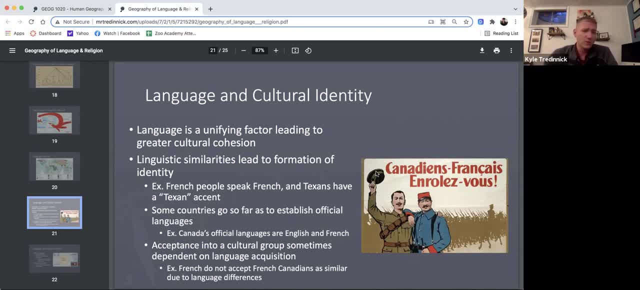 speaking French. Some cultures have gone so far, Or some countries have gone so far far as establishing formal languages or official languages. the United States is not one of those, but Canada has established English and French as their official languages. so on official documentation all throughout Canada, doesn't matter if it's Quebec or not. all official documentation. 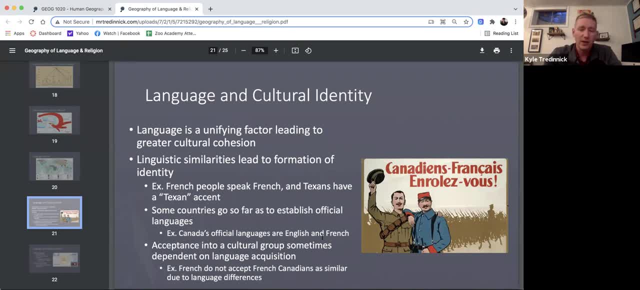 is in English and in French just because they have the those two official languages, and so what this means is that for incomers- people who are trying to assimilate or acculturate into that specific culture, they must also a lot of times, acceptance into those groups is connected to. 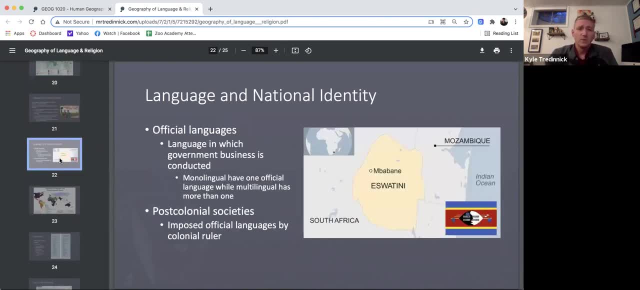 learning the language. so how we're, how we've been seeing this recently, is actually a really interesting one in respect to the continent of Africa, where Europe, during the colonial and imperial eras of the African continent, went through, divided it up, made their own divisions, and we'll talk more about this in. 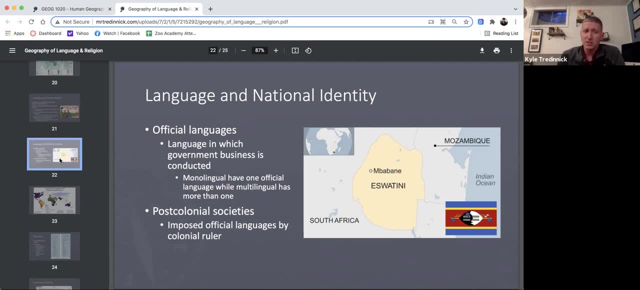 political geography. but since independence and since gaining sovereignty- which again is a concept we'll talk about here in just a moment or in a couple lectures here- a lot of cultures or a lot of countries have actually been going back and forth and changing aspects of the political affiliation and international recognition. 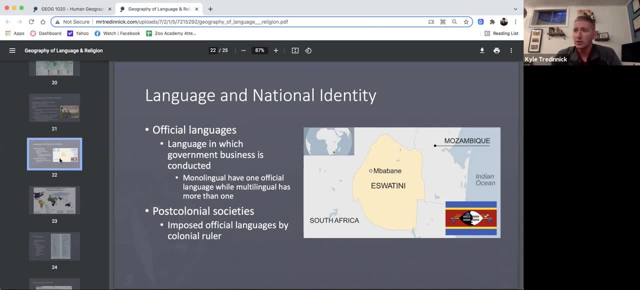 to more, to be more reflective of the cultural identities and language identities of that country. so the example that I have here is the country of East Watini, which used to be known as Swaziland, and it was just a couple years ago where they switched their language to be more reflective. 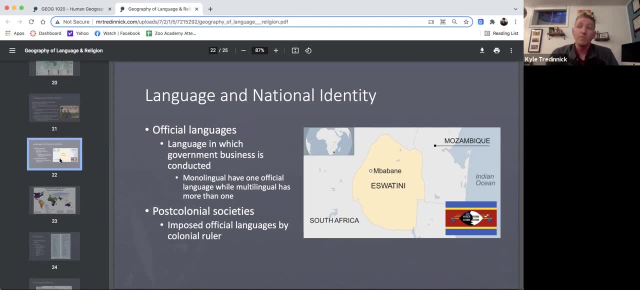 of their own cultural identity, and so I think that's a really interesting point and I think that's a really shared to show that It's from just a community as another one And but also in that sense of strategic Connectivity, another one here has been. there's actually 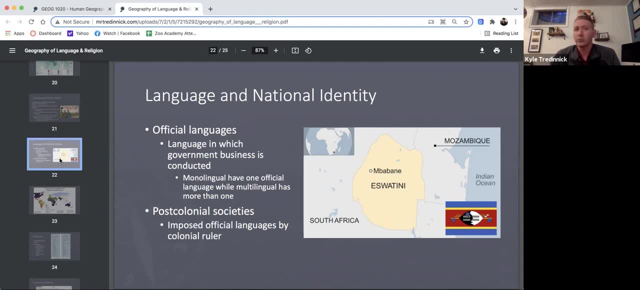 Telling Europe is the distinction of technique that, as a short form of the Czech Republic, You're instead of the Czech Republic is calling it check your Just because of the check probably kind of comes out of the whole idea of the check being one of the Eastern. 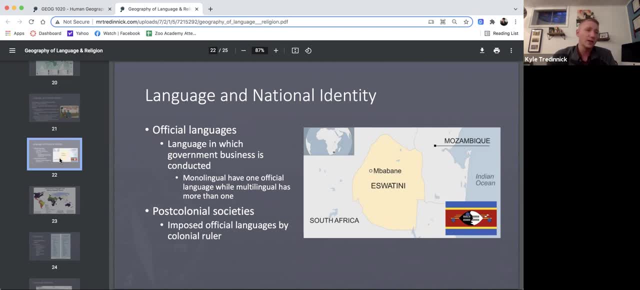 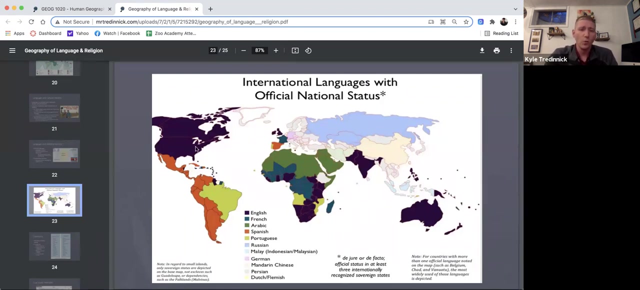 uh, even then it was the czechoslovakia, um, but being more reflective of the cultural understandings, recently, i believe within the last six years or so, um, they switched their name, or their short name, to czechia. so, um, official national statuses. so, yes, with these, uh, united states is not. 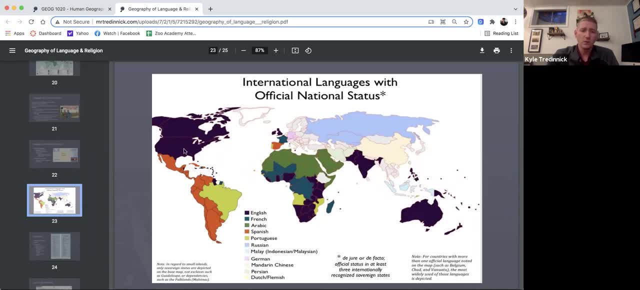 a official um or officially an english country, but it's a de facto country where, yes, we don't have an official language here in the united states, but all of our official documents, all of our official communications, take place in english, and so that's where that comes in. um. 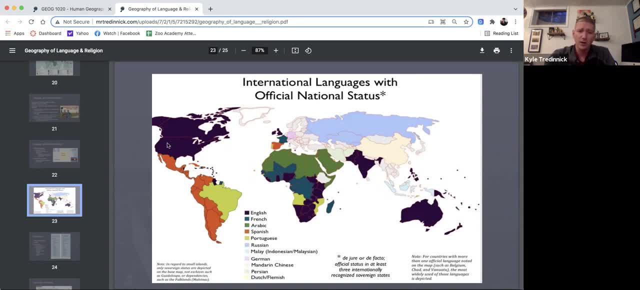 some languages or some areas don't have official languages, um, but then some very much do establish official languages as part of um what we call a centri, uh, centripetal force. it's something trying to pull the country together and they'll use a common language, um to try and tie that country together and we'll talk more. 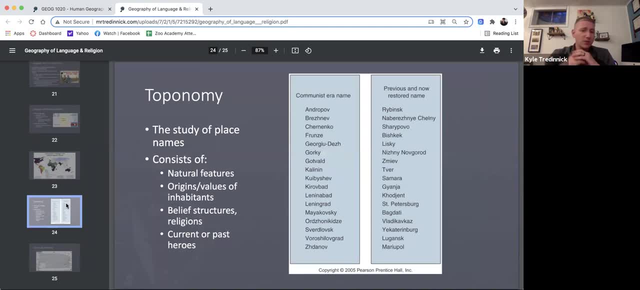 about that in political geography. all right, um, the last major concept here that we can talk about or look at when we're looking at language and we can see this reflected in the landscape, even though language very much is a, um, i can't think of the list. 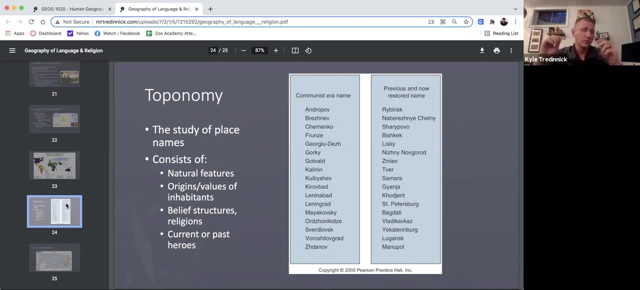 word off the top of my head here, an intangible thing where you you're not necessarily touching it, um, but one thing that we can see, and how language is reflected on the landscape, is through the toponomy and, uh, this is the study of place names. so where place names come from, these can 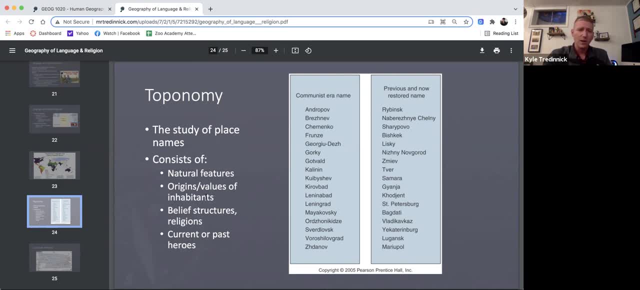 come from natural features. they can come from the original inhabitants that were there um. so, with omaha, the city of omaha named after the original inhabitants of the area that is now omaha, um belief structures or religious structures or current or past heroes. so washington dc named 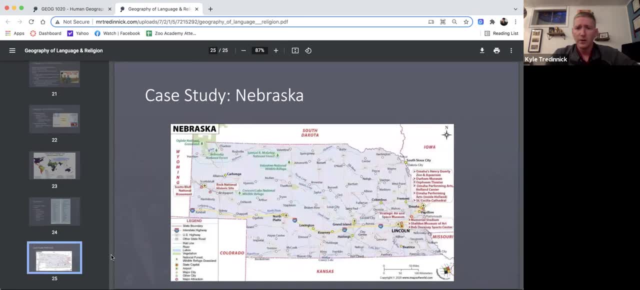 after george washington, so that type of thing. but if we look at omaha or nebraska as a whole, um a lot of it is connected to um settlers that came from the east and set up their own cities here, um some influence from the native americans who first lived here. so 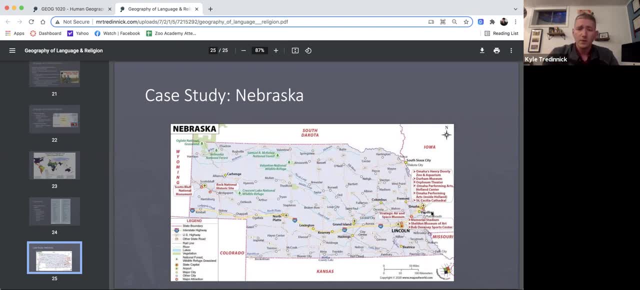 like omaha, um, so papillion, good example. it's reflective of so. papillion in french papillon is a butterfly, so it's a famous part of the monarch butterfly migration. so the name is reflective of the papillion. in french papillon is a butterfly, so it's a famous part of the. 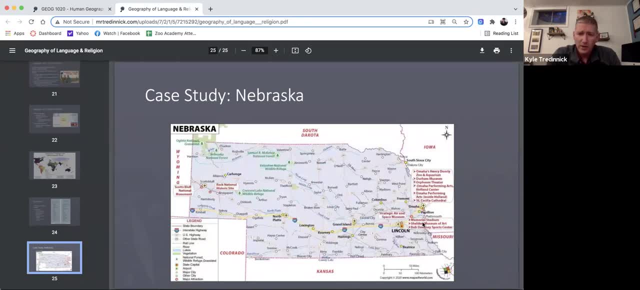 national park and it's a nice part of the national park and it's a nice part of the national park um. so um, it's a kind of a very interesting kind of that natural behavior or that natural um connection. and then let's see here some other good examples um dakota city named after the 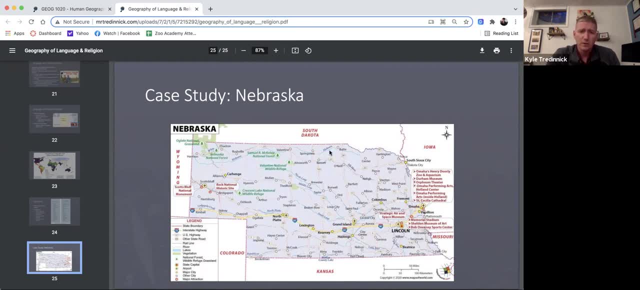 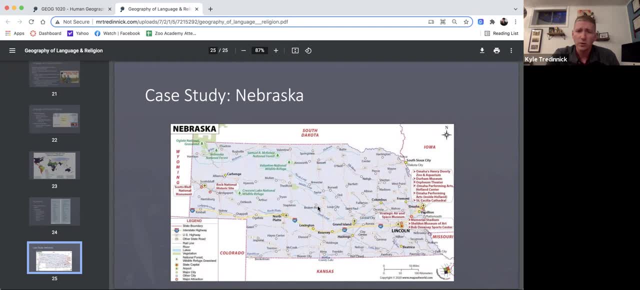 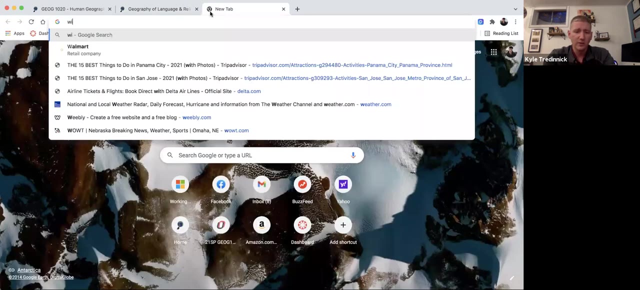 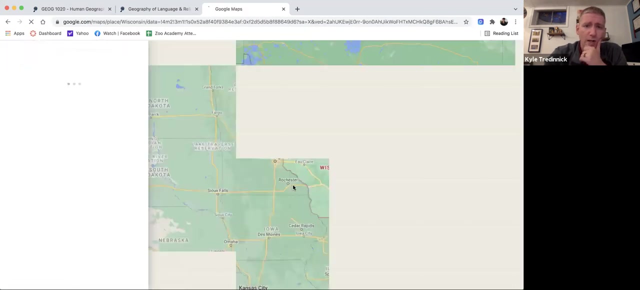 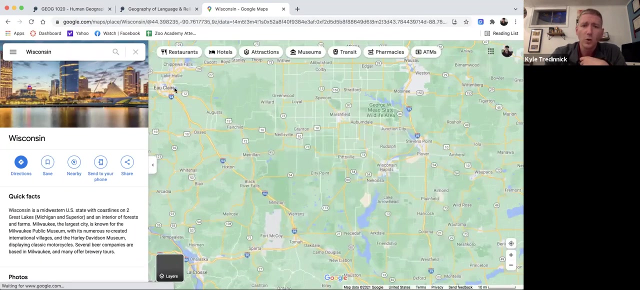 I would mostly say pot or connection to native name to that. So yeah, just looking at this, Nebraska doesn't have necessarily as much as when we go to. Let's go to the state of Wisconsin And if you pull up Wisconsin here we can go in And there's a lot reflected in Wisconsin with Eau Claire heavily French influence. the nominee. 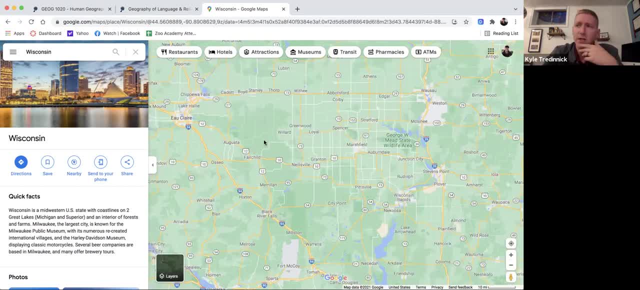 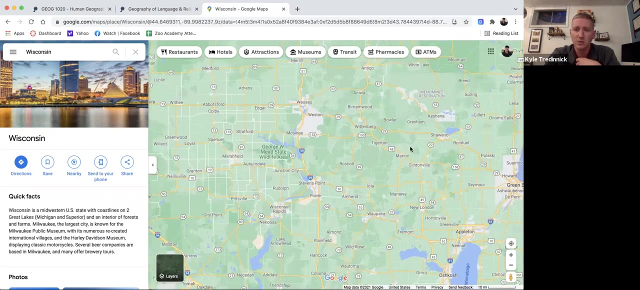 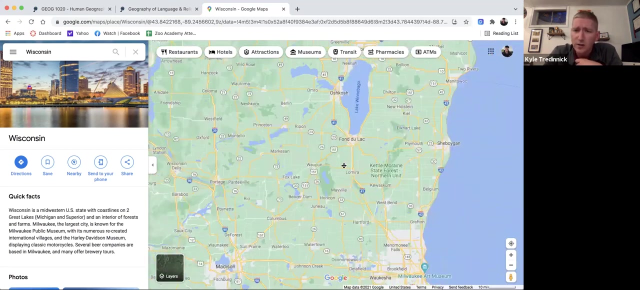 So heavy influence on the early sock Fox, Ojibwe or a cinema line. So Wausau nominee, there's the nominee reservation and you see those names reflecting on the names of the cities itself. I'm trying to find there should boy again. 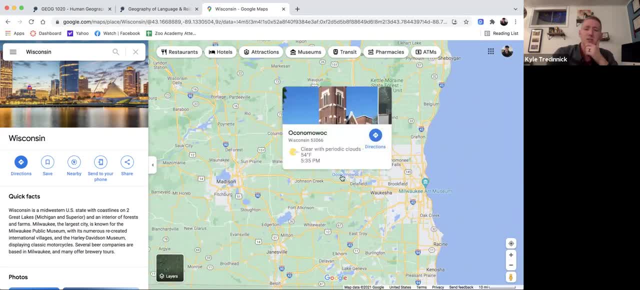 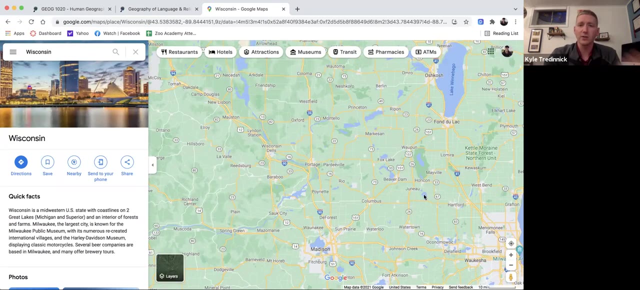 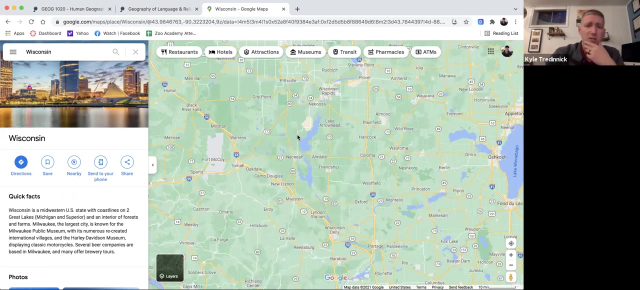 One of the most fun There. it is One of the most fun city names to say in the country, kind of a walk, walk, a shot, Um, so really reflecting the heritage of the native people, the first settlers and some of the European explorers, the first settlers and coming from the east. 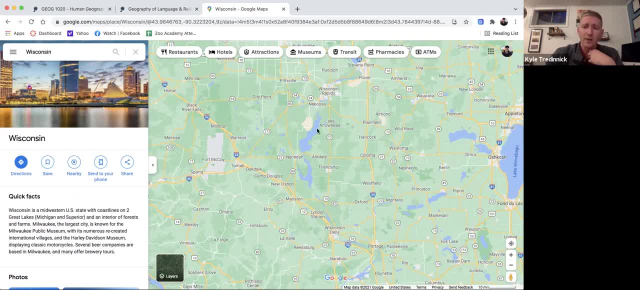 Um, so a lot of that showing up in the topography or economy of Of Wisconsin itself. So, um, that really covers language and religion, And so next we'll look a little bit more at culture and then move into political geography. So thank you very much for joining me.